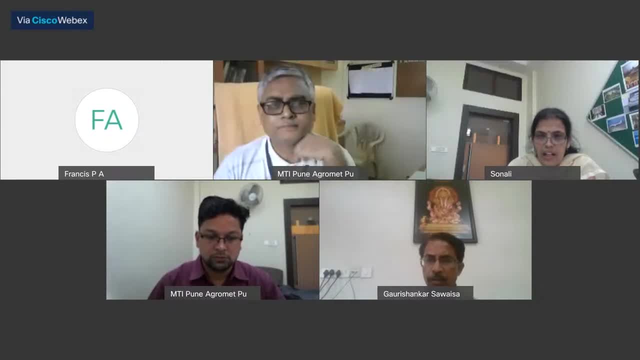 Office of Head CR&S. I would like to request Dr Sunad Dutta, Sir Head MTI, to brief about this new initiative of webinar series started at Met Training Institute, Pashan Pune. Thank you, Sonali. Actually, Meteorological Training Institute, it is the main center of India Meteorological. 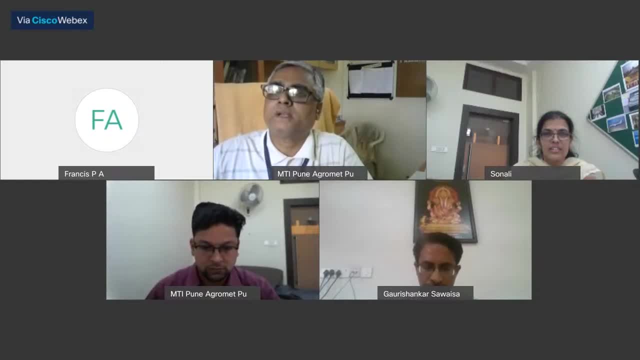 Department for the capacity development of meteorological personnel of the department, extra department and overseas participants in the field of weathers and allied services. Till now, this training institute has been the main center for the capacity development of meteorological personnel in the field of weathers and allied services. 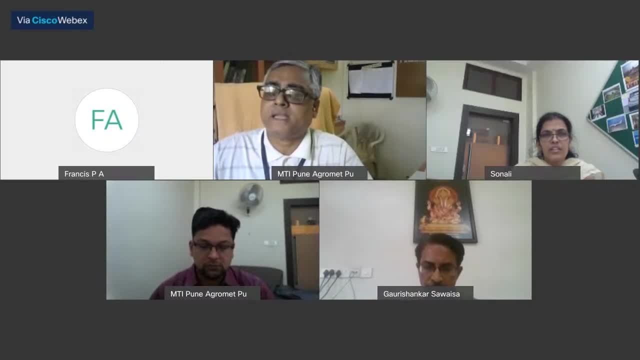 So this wings of India Meteorological Department is engaged mainly to strengthen and develop the capacity of the meteorological personnel in the field which I have mentioned. But now it is a societal demand that training wings of India Meteorological Department should take the responsibility. 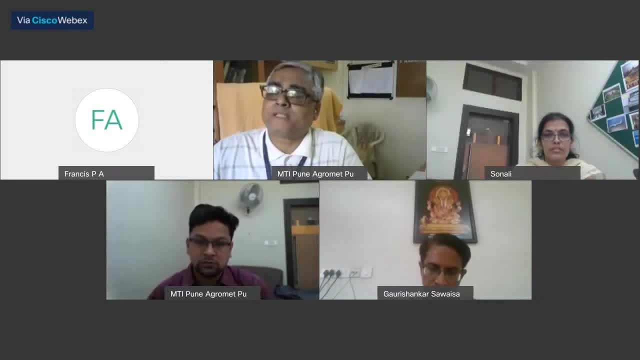 The responsibility of developing the capacity of the community also in the weather services and the allied services, also weather and climate services and allied services. In view of that, DGM IND has, kind enough, he has entrusted upon this new assignment to this Meteorological Training Institute. 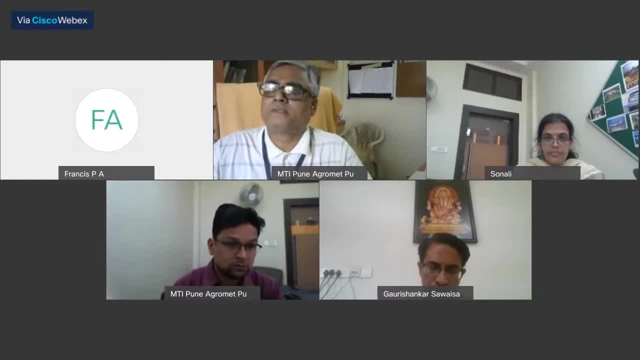 And we thought how to achieve this goal. now, to achieving this goal, we have started this new initiative of organizing webinar series of lectures by eminent scientists, operational meteorologists, which will help the community, general public, media, all those people who, all those people in the field of weather services, climate services, etc. 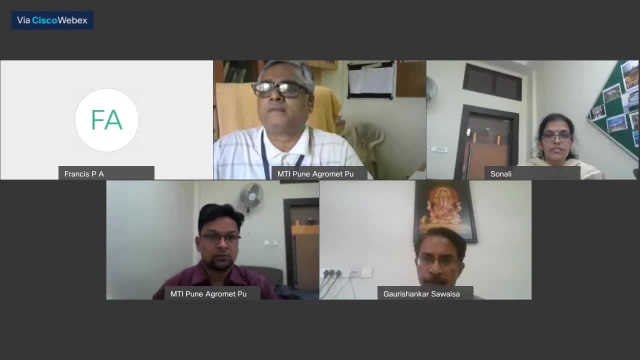 Thank you very much. our invitation. I now request Mr G K Savaisarjee, scientist, to say a few words about Dr Francis. Thank you, Mr Savaisarjee. you are muted. You speak from the beginning. 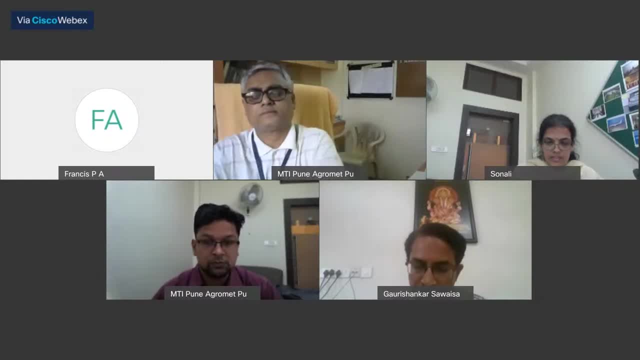 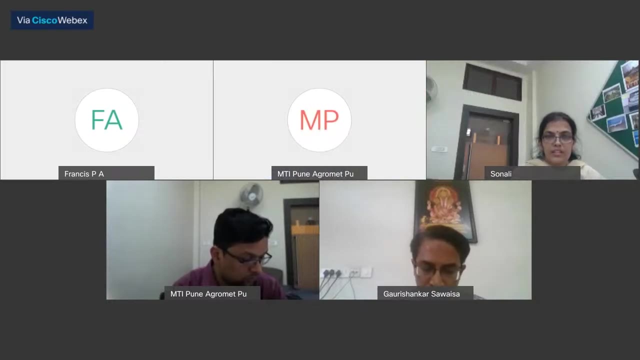 I am really honored and happy to introduce today's speaker, Dr Francis, scientist at affiliated to Indian National Center for Oceanic Information and Services and the Ministry of Earth Sciences, to meteorological fraternity and viewers. He is head of Ocean Modeling and Data Assimilation Division. 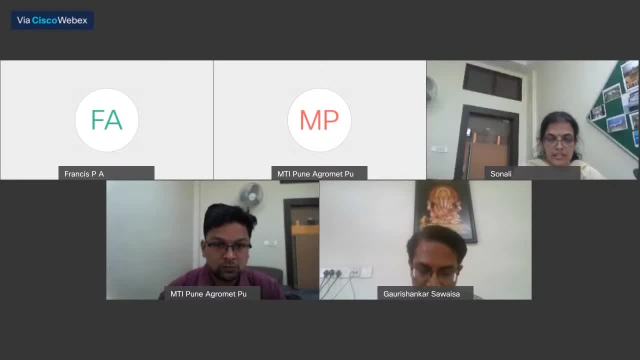 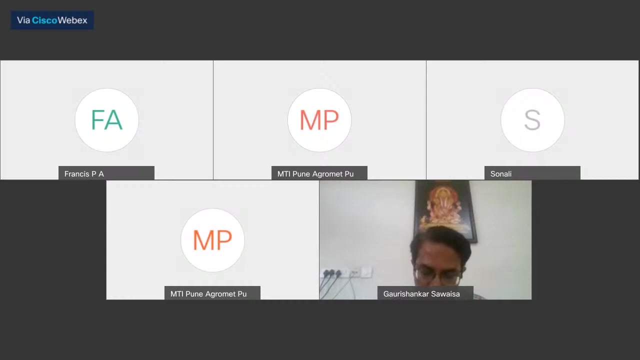 He is Project Director Mansoor Mission Phase II. He is Chairman Academic Advisory Committee for International Training Center for Operational Oceanography and Students Coordination. His research interests are numerical modeling of ocean general circulation, waves and tides. Indian ocean variability. Indian summer monsoon variability. coupled processes over the tropical 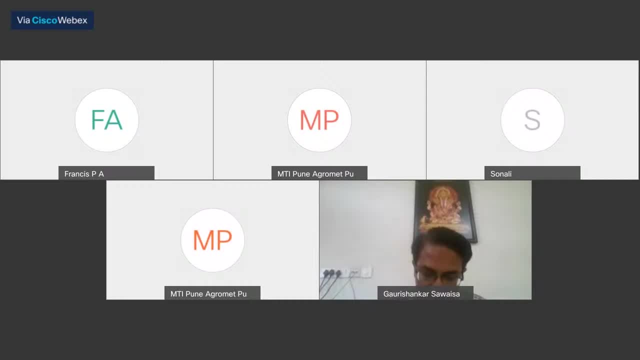 oceans. His credentials are: number of papers in peer-reviewed international national journals are 38, number of chapters books is seven. and he has many awards received and among them, in 2010,, he has received MOES MET Certificate Ministry. 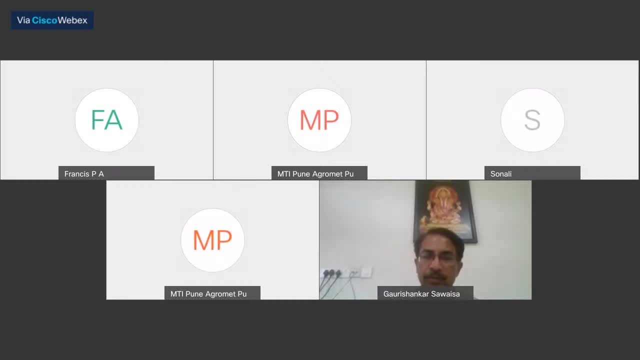 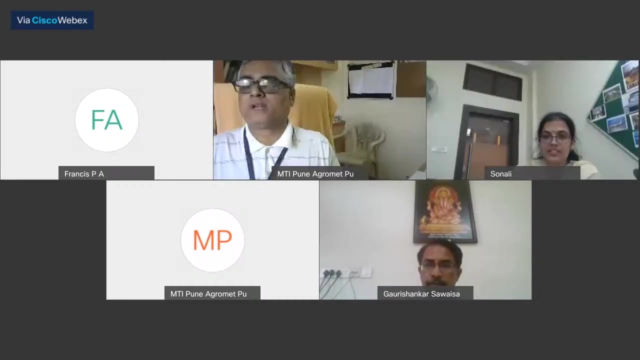 of Earth Science Government of India. Thank you, sir. Now I request Dr Francis to give his WMO talk- WMO Day Talk. Thank you, Dr Somana, Dr Gauri Sengar and others. Are you able to hear me? 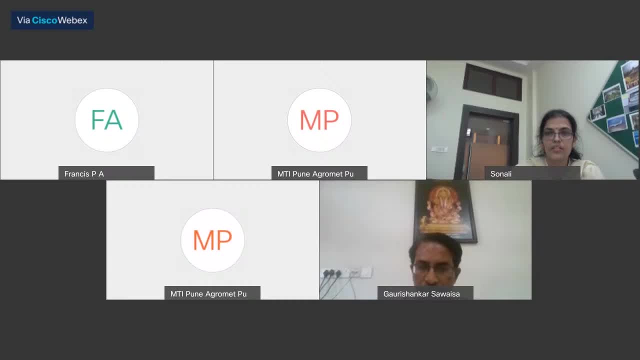 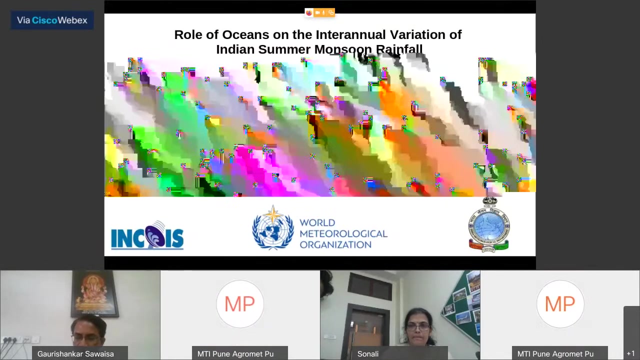 Yes, sir. Okay, So thank you very much for inviting me for this important event. I will share my slide and from there we'll start. Are you able to see my presentation? We are able to see. We are able to see. 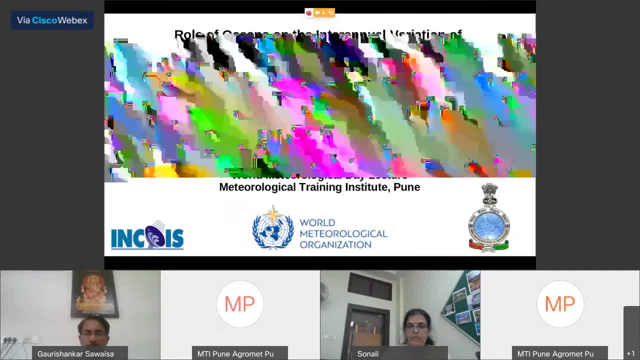 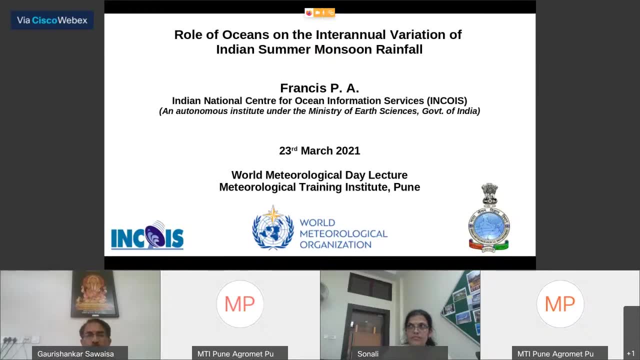 Okay, Thank you, Dr Somana. Okay, So today I will be speaking on the role of oceans on the interannual variation of Indian summer monsoon rainfall. Okay, Yes, Thank you, Dr Somnath. 3rd of march 2021, the world meteorological day, and we know that this year, wmo has dedicated. 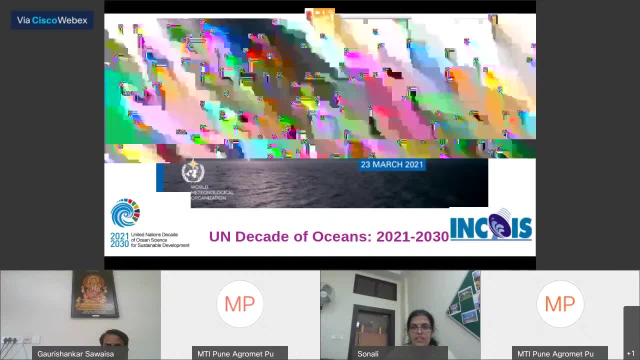 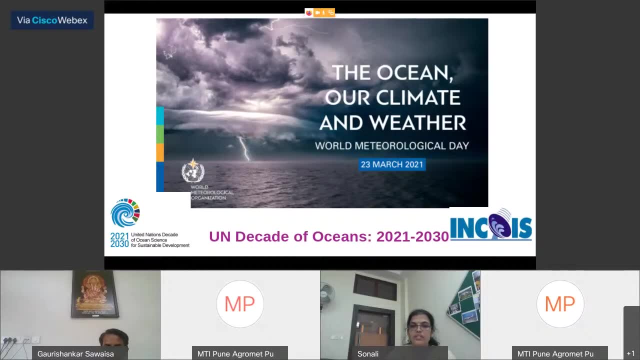 the world meteorological day to the oceans. the theme is: for the oceans, our climate and weather. this marks the beginning of 2021, marks the beginning of even decade of oceans, the next 10 years. wmo and intergovernmental oceanographic panel commission has decided to spearhead the activities on ocean research which we can, you know, use. 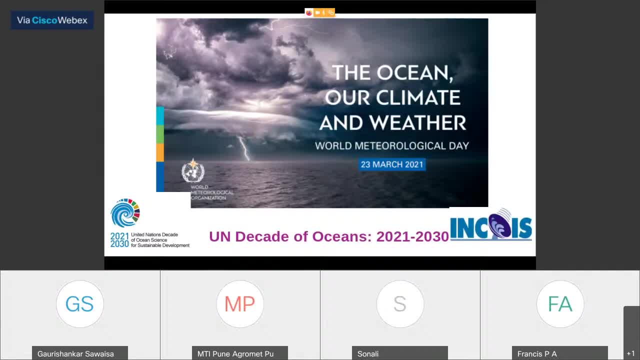 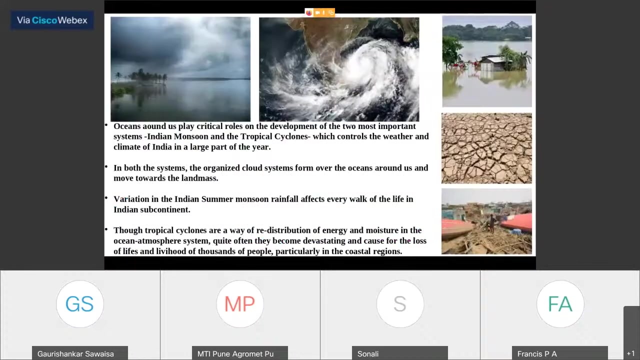 to harness the fruits of ocean sciences for the sustainable development. so i thought it's a appropriate. when we talk in india, it's appropriate to talk about the role of oceans on indian monsoon, which is the lifestyle of our country. when it comes to india, we talk about two major weather systems. one is the eastern monsoon system and the other one is 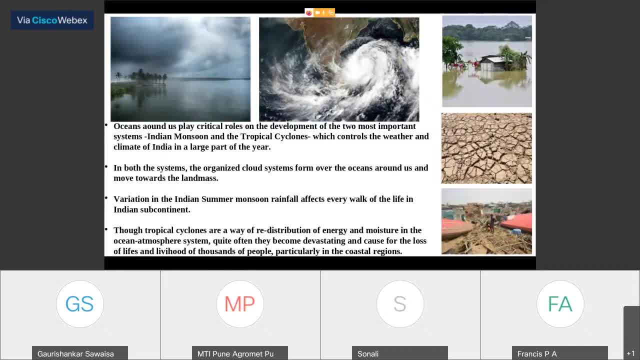 the tropical cyclones. these are the two uh ocean, uh related or something which has strong connections with oceans and affect the life and livelihood of our country. so so ocean plays an important role in the development of these two systems, because these two systems get energy and moisture uh from the tropical ocean. most repairs for tropical oceans. 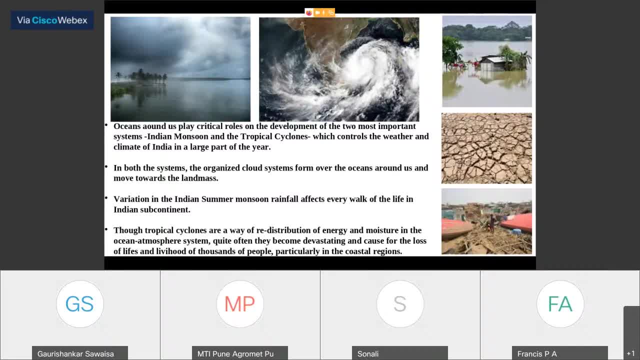 both the systems are organized, knit and we know that. the way there is considerable variation of rainfall, what we get in the indian summer monsoon season- and this affects every walk of life- or in our country and the neighboring countries, for example, floods, droughts and devastating cyclones- affects our everyday life. 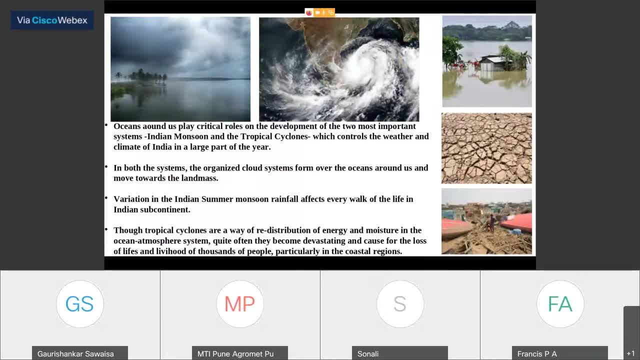 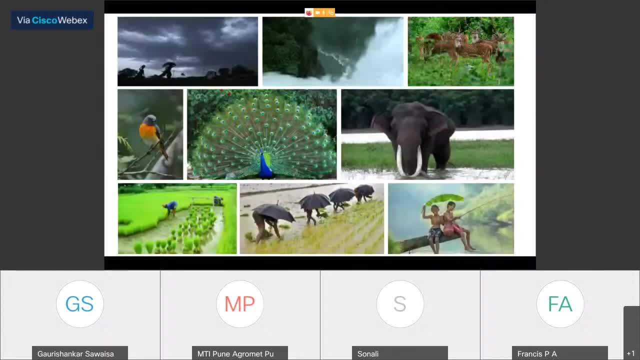 when it comes to. well, now, for those who are interested to follow the monsoon, the first thing which we always talk about is the arrival of monsoons at somewhere in the southern tip of india, kerala, with very deep, thick black clouds spreading over a large area and start giving. 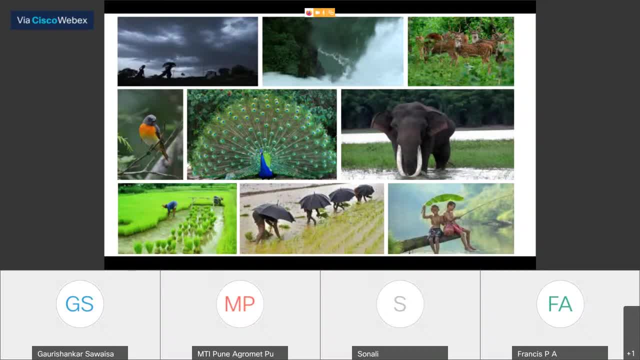 rain, and this rain set the mood of the nature also, and all animals, birds, plants, everything changes it's life pattern to in tune with the rainy season. and we also know that a large fraction of our agriculture is still rain first. so we have our agricultural calendar tuned to the arrival. 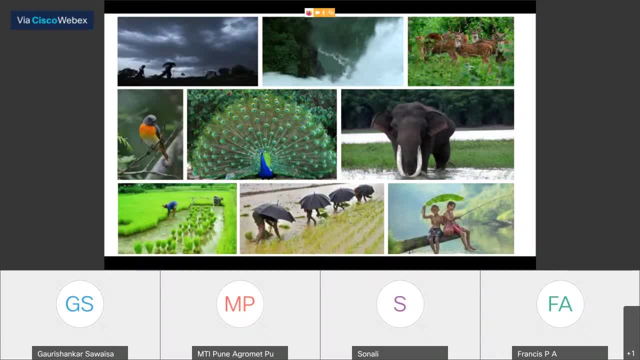 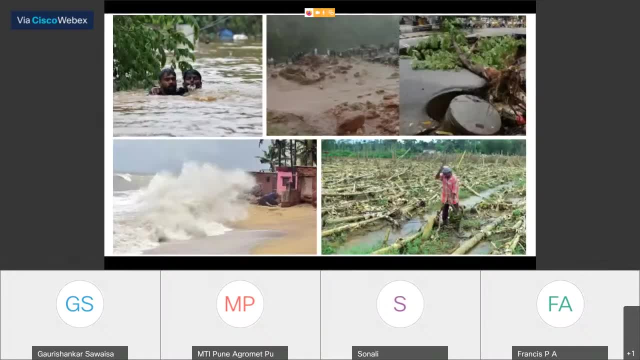 of monsoons and of course, it's a fun time for kids too. but it's not always very fun when we talk about monsoon. monsoon- if it's very intense, it can affect the life in form of floods, landslides which can wash away the villages or, you know, settlements. it can destroy our infrastructure. 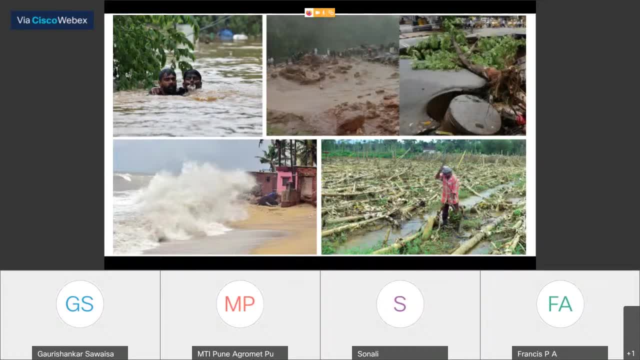 uproot trees. coastal erosion is an important problem which we may come across during the monsoon season, and the coastal bench and loss of livelihood is something which is quite common when it comes to- uh, you know- heavy rain, apart from droughts, which can also have serious impacts on. 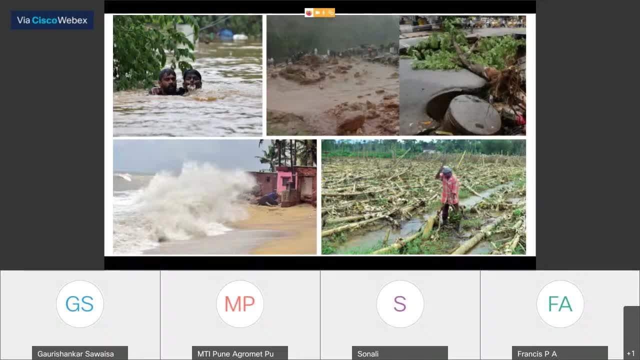 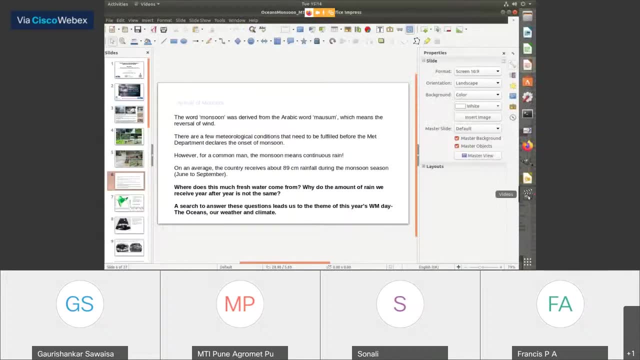 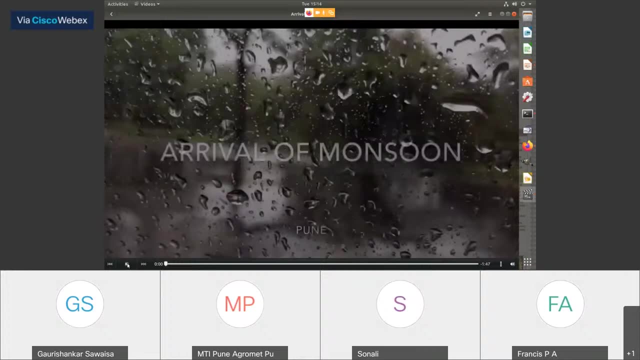 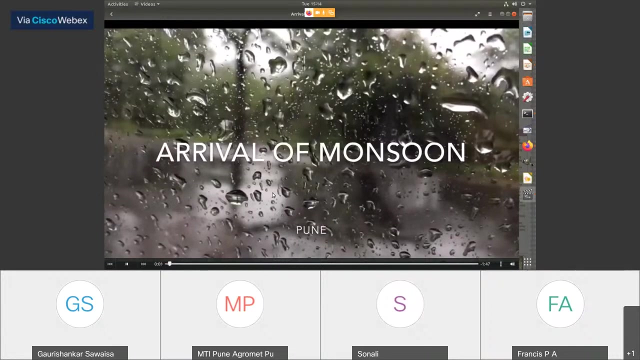 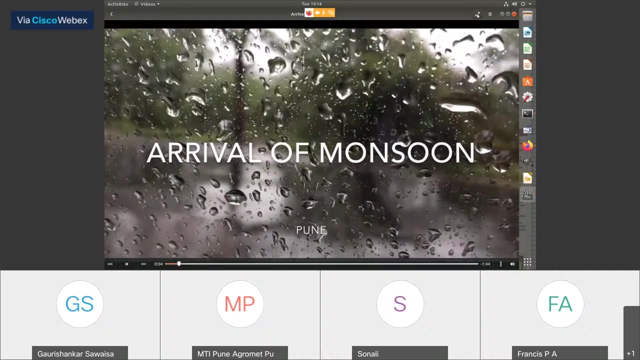 our agricultural activity. so i will uh quickly play a small video which i have taken from youtube just to set some of the speed, so i hope it is visible to you, and it just marks how we get rain during this monsoon season and those who are following the monsoons and those who are monsoon. 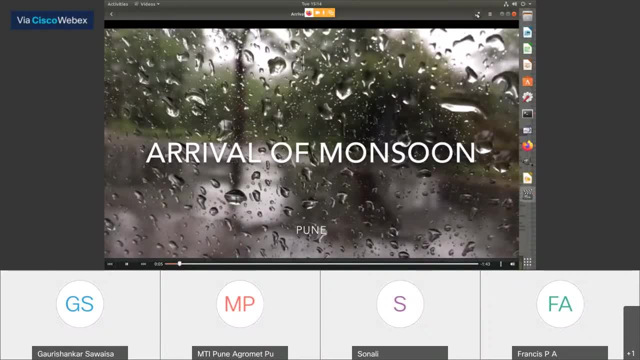 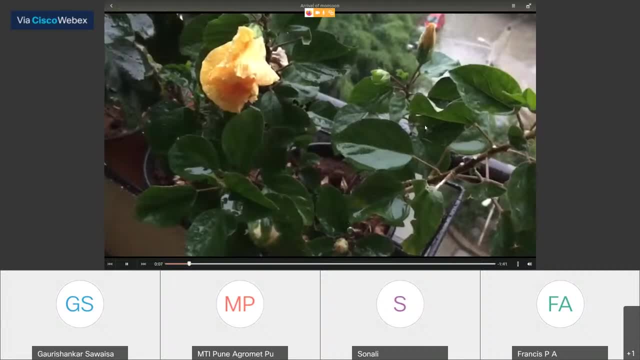 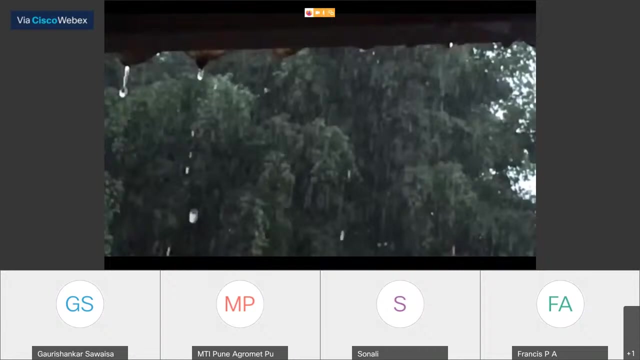 lovers must be very familiar with the way we get rain. you know starting from small bristles to. you know large, you know showers. it's something which we always wanted to have. so this is a short video. it's, uh, just for two minutes or less than two minutes, and we can say that the rain 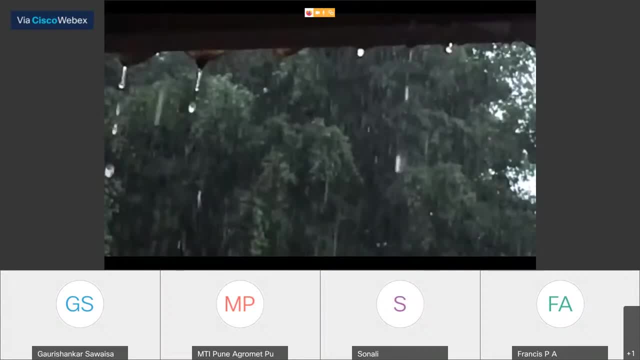 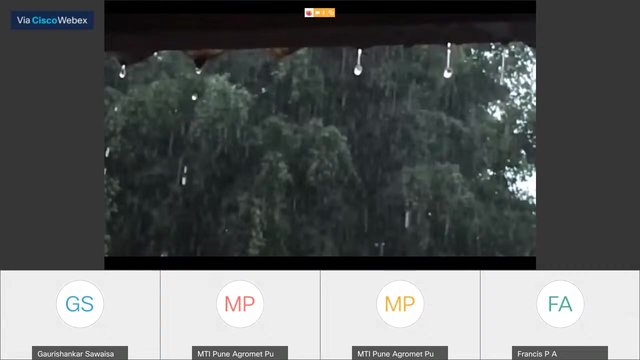 that we receive during the monsoon season gives the fresh water very much required for the life to thrive in the subcontinent and that's how the monsoon help us. so monsoon rain that happens over the- um, you know, hilly area in that, uh, california, who can have the tight beside. the timing of the monsoon is, i believe, um six percent, is two percent long for that, kingarde im5 floating cascadro uproot. 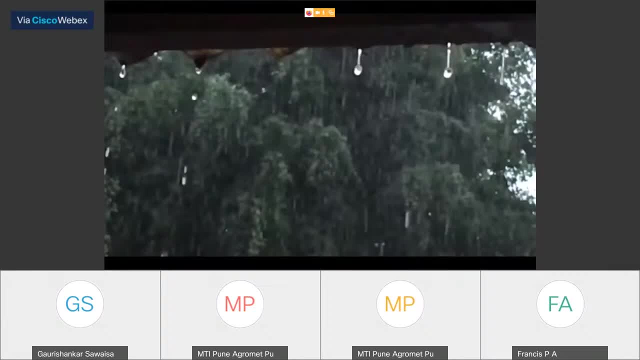 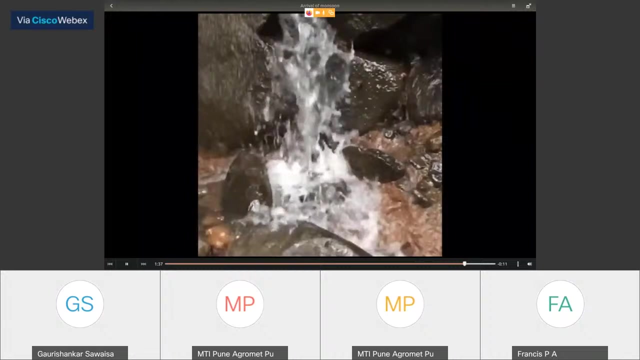 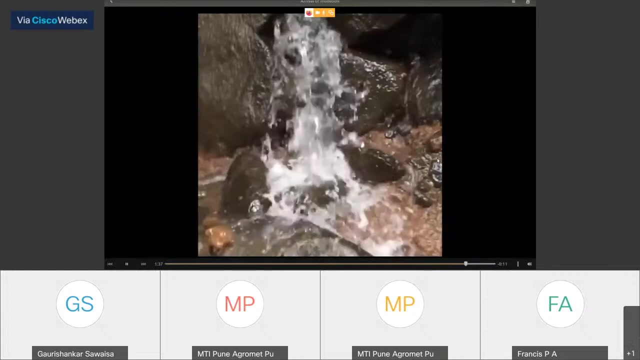 areas are going to give the required water, fresh water for the rivers to flow, mostly in the Western Gulf region and other parts of the country. This is a very important process. Okay, so I hope that sets the tone of the remaining slides. Now we all know that the 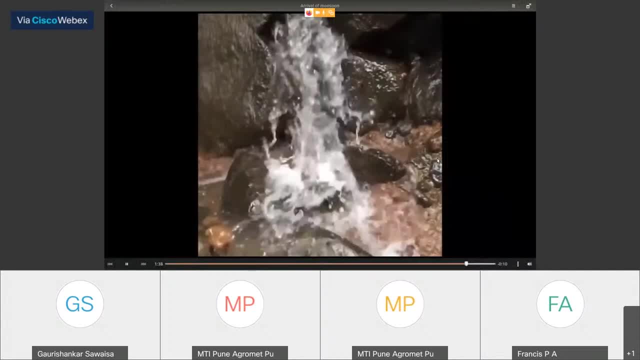 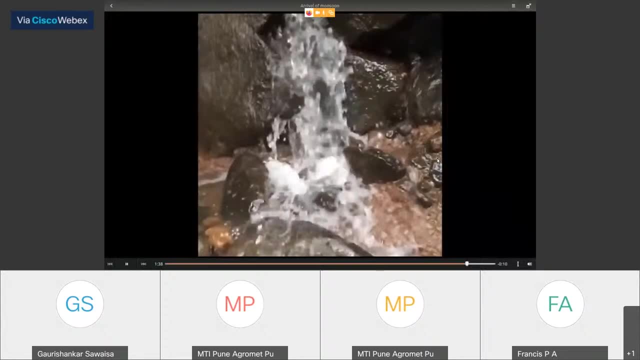 word monsoon was derived from the Arabic word Mosum, which means the reversal of wind. And when the MET department declares the onset of monsoon, it's not only the wind, but many other parameters also are considered before finally declaring the monsoon. But for a common 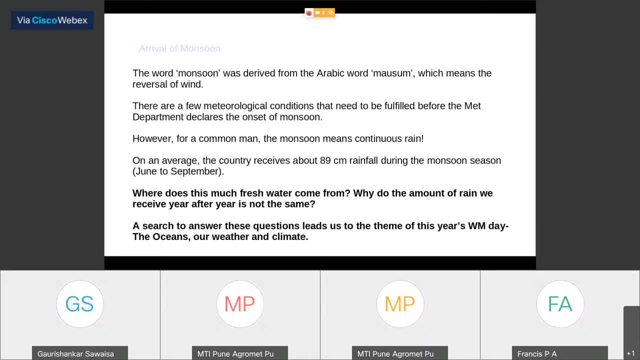 man who looks for the monsoon. the monsoon means continuous rain and rain and rain, which is the monsoon. This is going to be the most important event in the monsoon season. In a monsoon season, even if we have good winds and if we don't have rain, common man is not going to be very 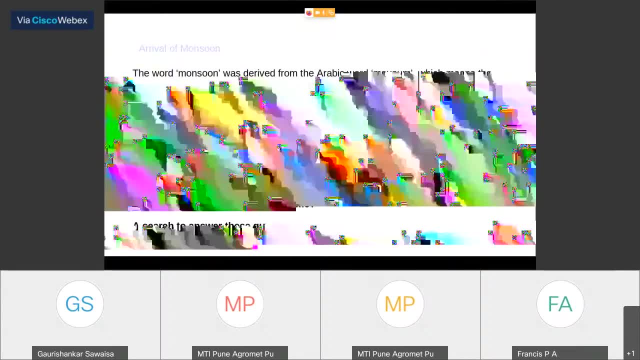 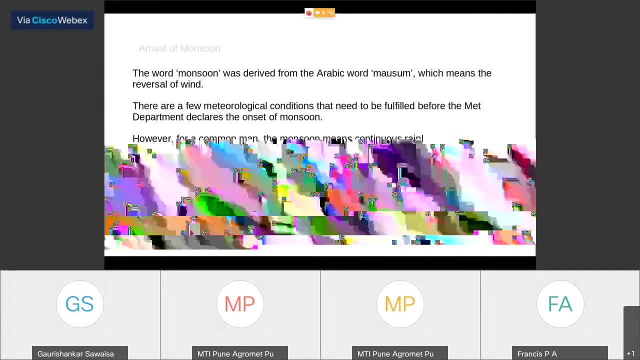 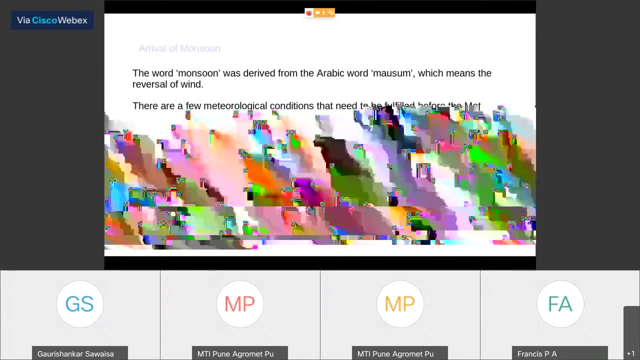 happy. On an average, the country receives about 89 centimeter rainfall for the entire four months of the monsoon season. The question which immediately comes into our mind are: where does much fresh water come from, And why do the amount of rain we receive year after? 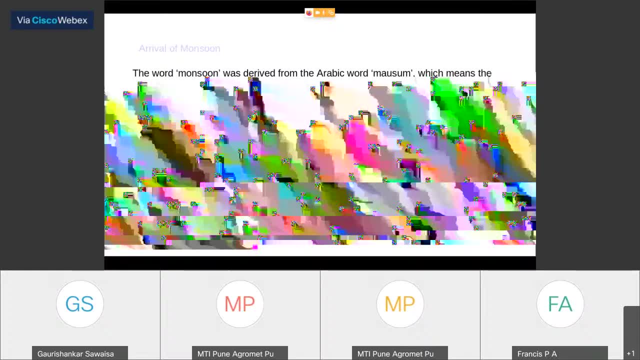 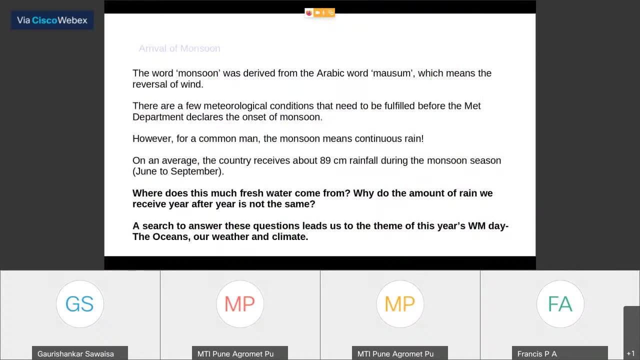 year is not the same. If you try to answer these questions, I think we are close to the team of WMO Deceleration in 2020.. Now, if we are looking for the spatial distribution of rainfall, Okay good, There is nothing yet. 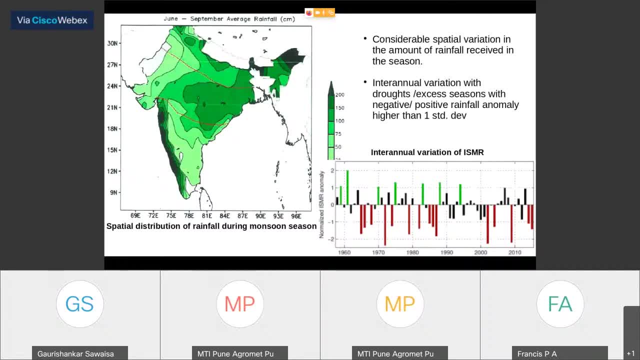 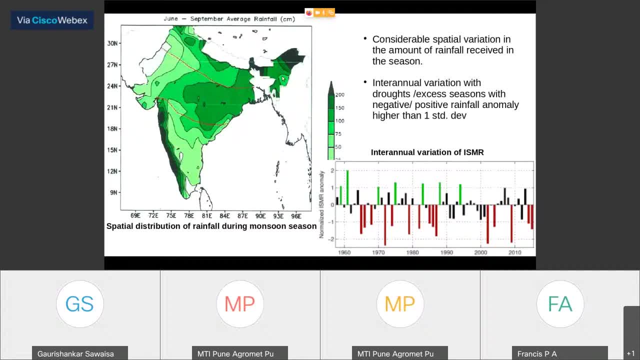 the western Ghat region. We have very good rainfall over the northeastern parts and also to some extent good rain over the central parts of India or eastern parts of India. But rainfall distribution, if you look at carefully the northwestern part and southeast- 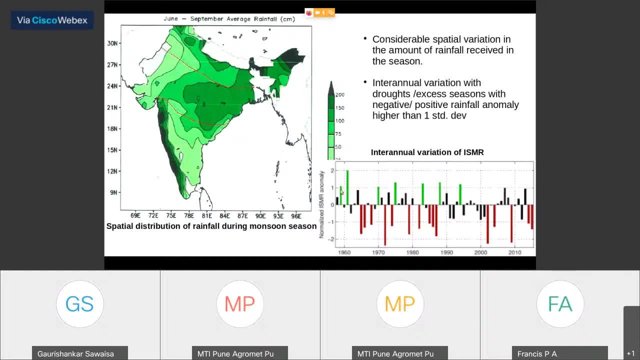 part receives less rain. And if you look at year to year variation of rainfall, you can see that there is considerable variation in the rainfall and there are years in which the rainfall goes. you know something like about one standard deviation from the mean. 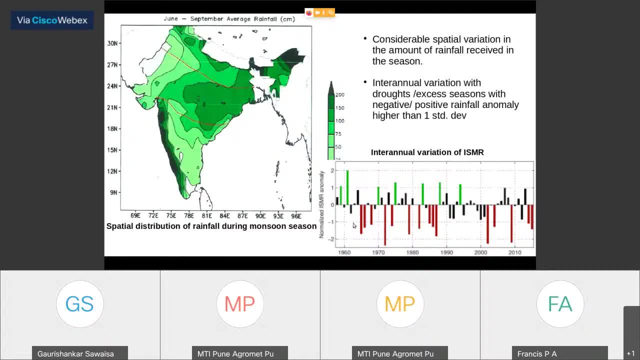 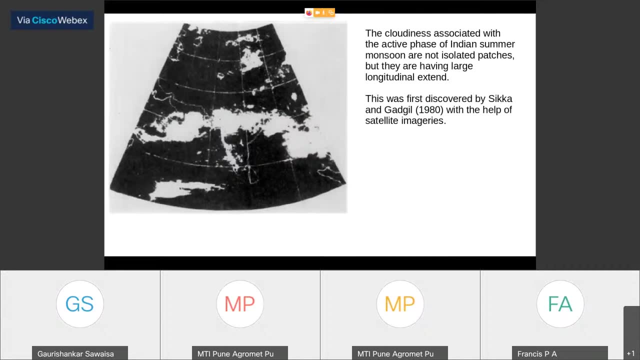 line which we generally call as excess seasons, And there are years where the rainfall is below normal by one standard deviation or more, which we call as droughts. Now, earlier research by Sikka and Gardgill in 1980 has brought out a very important aspect of monsoon. 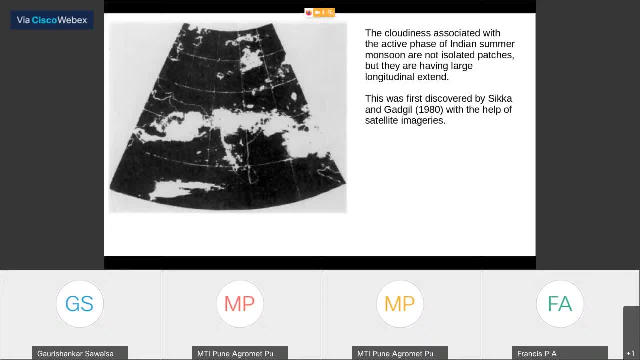 that the rainfall that we received during the monsoon is not coming from isolated cloud systems, but rather it's coming from a large-scale organized convective system. They have done this with the help of satellite imageries, which were very rare on those years, But they 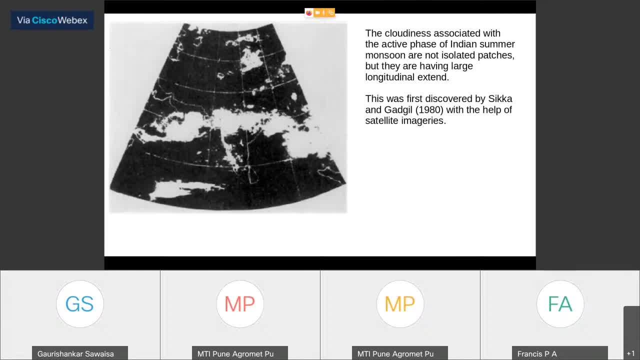 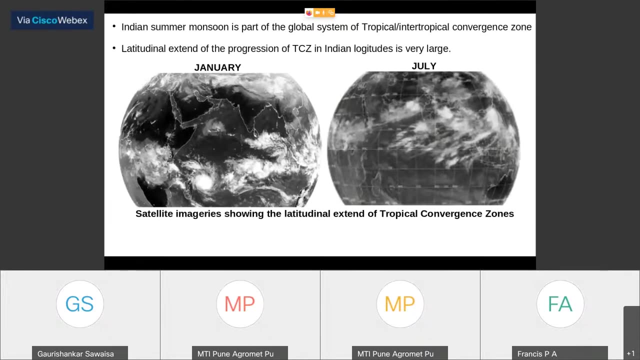 years. but continuous monitoring of these satellite images give them an impression of how large the cloud systems are during the monsoon season. but if you look at the global picture of cloudiness we can see that it's not just limited to the indian region. it has large like a longitudinal 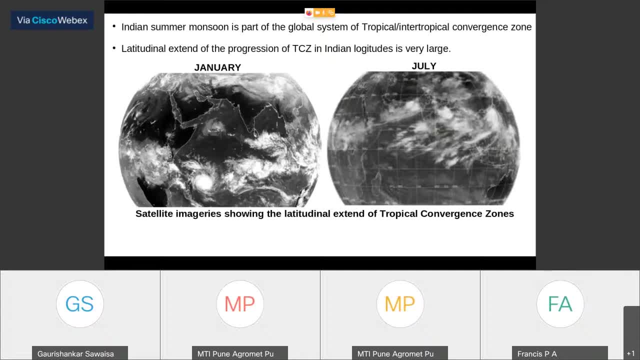 extent it- it's almost seen across the globe and also it's an important factor that we may come across when we analyze these satellite images- is that there is a large latitudinal extent or latitudinal variation in this cloudiness from january to july. 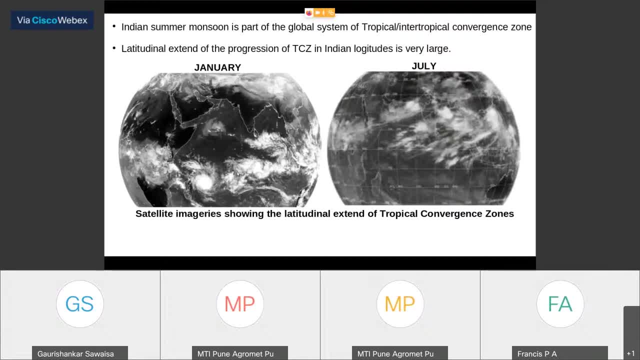 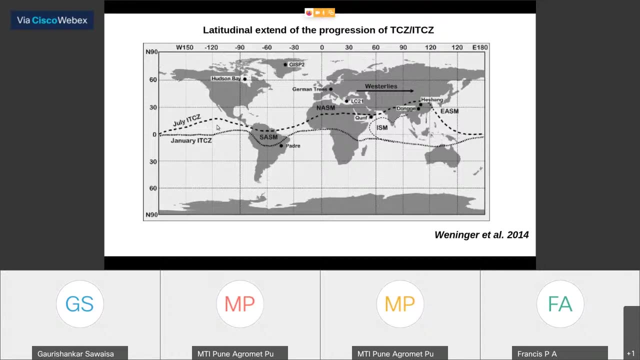 when we look at this satellite images, so our indian longitudes, these are having this cloud systems migrate quite a lot from january to july. you can see that more clearly in the picture where the mean location of intertropical convergence zone is located during july. 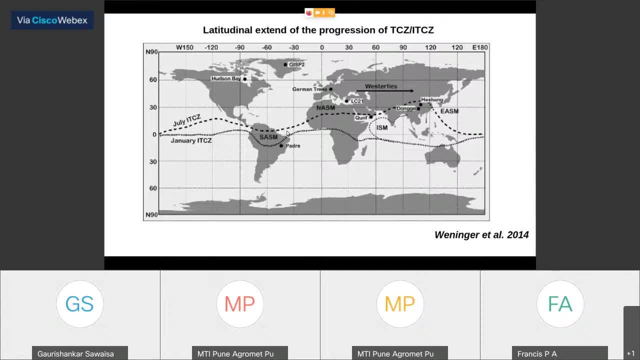 and january, you can see that most part of pacific and the tropical atlantic, the january and july itc sets are close by. but when it comes to the indian region we have a large uh latitudinal extent or which this january and july atc set are separated and 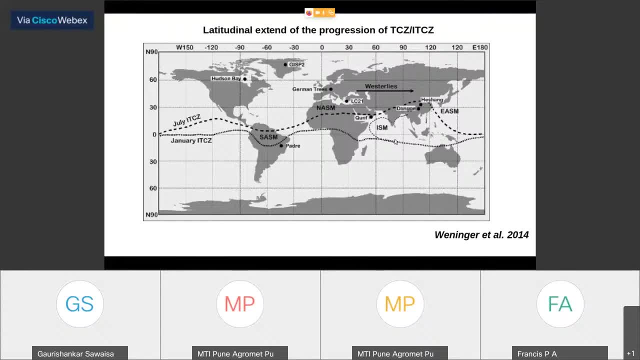 also, when it comes to the indian region, we can say that it's not the- uh, you know- moisture laden air that come from the southern hemisphere that converges at the location of the convergence, but it can be from the same latitude itself. so often they are referred as tropical convergence zones. 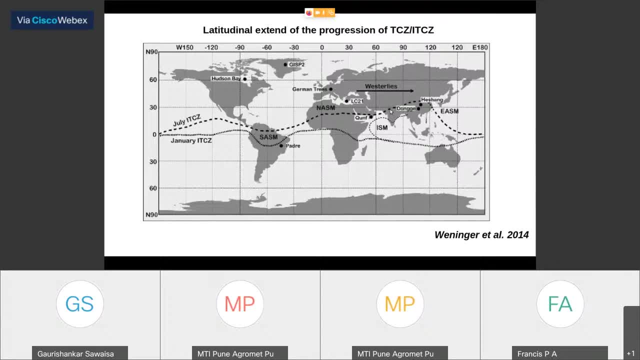 instead of intertropical convergence zone when it comes to the monsoon regime. so if you look at the rainfall in the uh tropical oceans in the indian region, then you can see that the indian region is oceans near us, the top panel. you will see that the rainfall that we get during the monsoon June. 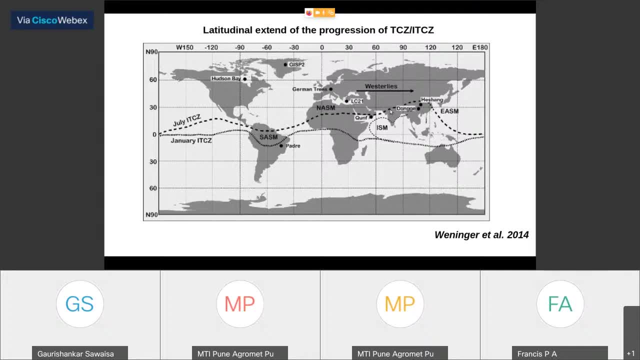 to September season. there are two peaks you can see. One is near the equator, which we can call as oceanic T-season, And then of course we have a northern part also, And quite often you can see that during the monsoon season you can see that cloud system which you can see in the right-hand. 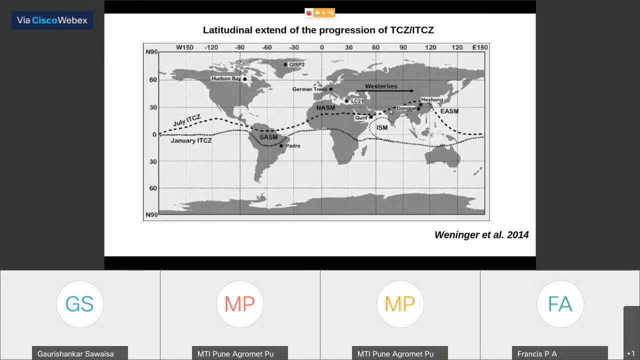 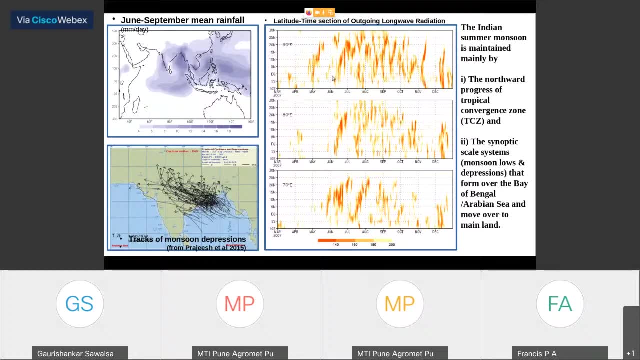 side. what I have plotted is the long-wave radiation, outgoing long-wave radiation, which is plotted as a function of latitude and tide. Outgoing long-wave radiation is a very good measure of cloudiness: lower the values of oil, higher the amount of cloud we have. So you can. 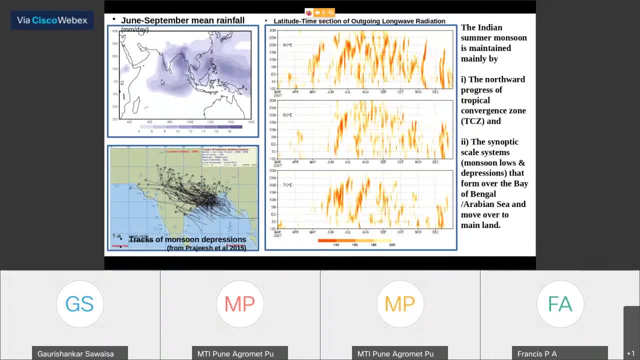 see that from the equatorial or oceanic T-season, where the oceanic T-season is present, we have a lot of cloudiness, So we can see that from the equatorial or oceanic T-season, where the oceanic T-season is present. from there to the northern part there is a migration of a. 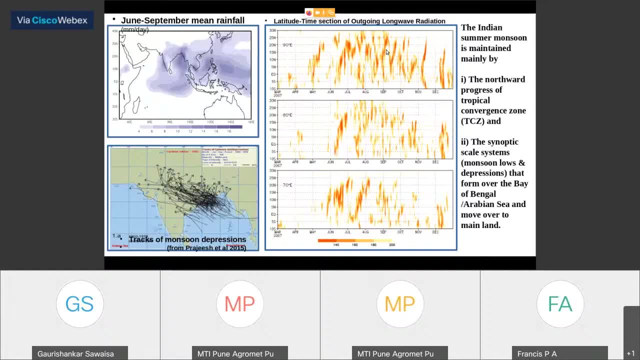 T-season Quite often. that happens, probably two or three times in a season, And the latitudinal extent to which the northern part to which this T-season extends varies. During June it goes to something like 20 degrees, But when the monsoon is completely set over the country, 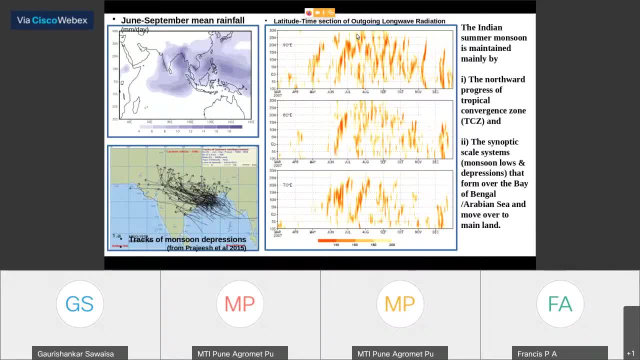 in July and August this can go up to 25 degrees or even more, And when the monsoon retreats, you can see that same kind of northward propagation happens, but they are limited to a lower latitude. So this is how the oceanic T-season is feeding. 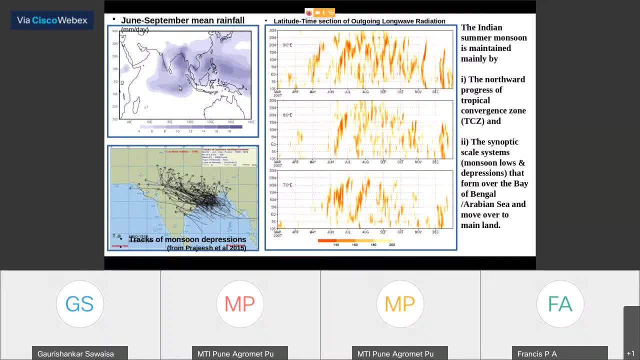 to the continental T-season or we can see that how the monsoon is progressing in terms of T-season, But monsoon is maintained not only by T-season progression of T-season, but also by the low pressure systems and monsoon depressions which form over the warm oceans. 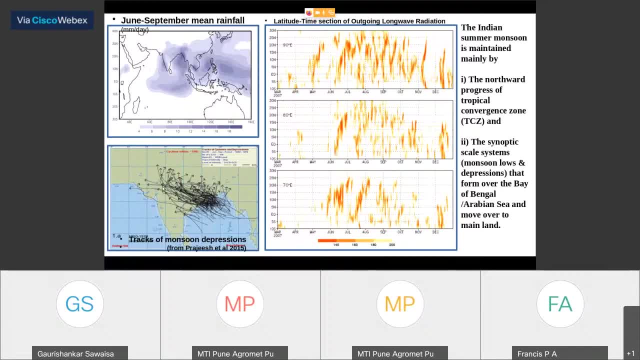 Like Bay of Bengal and the South China Sea, and then move over to the Indian mainland. So there is very much a good connection between the rain, what we receive over the land during the monsoon season, and the processes that are happening over the oceans, So maybe understanding that processes. 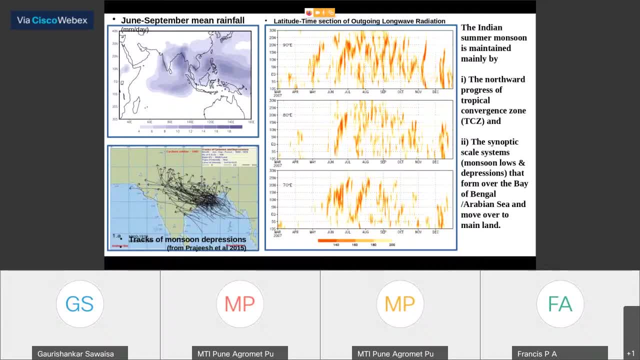 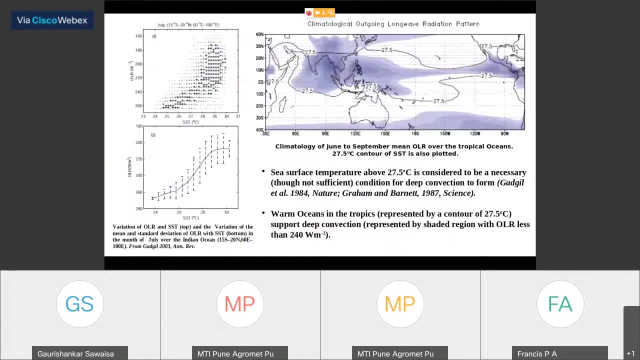 those processes will give us a clue on how the large scale variability in the interannual timescale is dependent on the ocean part. Now for those who are very familiar with the ocean atmosphere process, the most important parameter that interacts between the atmosphere and the ocean is the sea surface temperature, because it's on the boundary of the air-sea interface. 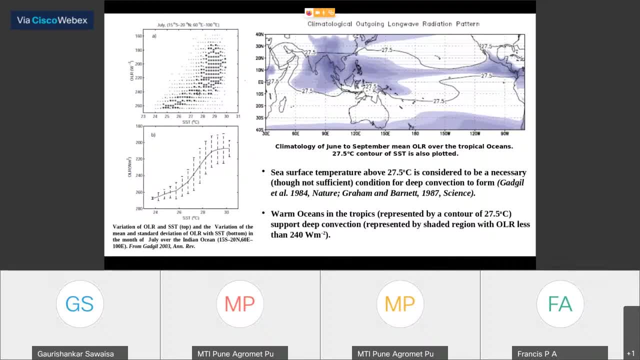 And we have a good research And there are two classical papers which talk about the relationship between the sea surface temperature and the deep convection. Godgill has shown in the 1984 that a temperature of about 27.5 degrees is a must for deep convection to form over the 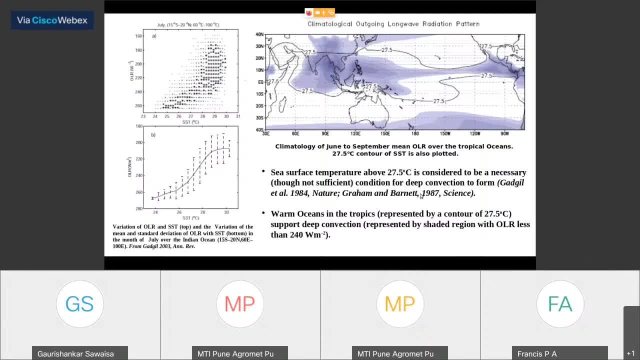 tropical oceans, And Graham and Burnett also have said that 27.5 degree is a good threshold, but that's not the only condition that is required to have the convection. Now, if you look at the right-hand panel of the screen, you will see that there is a special 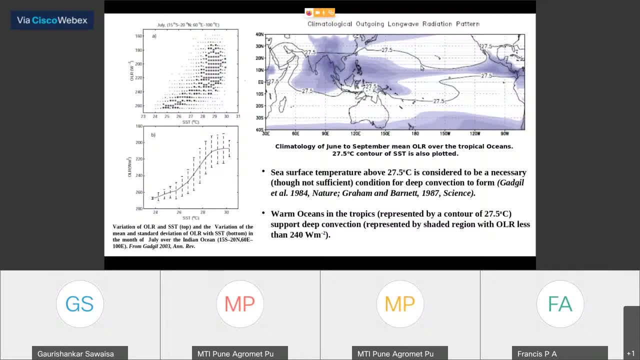 pattern of outgoing longwave radiation. It's a climatological pattern for June to September, And then there is a contour that encompasses 27.5 degree isotherm. You can see that the convective regime, which is shaded part in that map, is completely enclosed by the 27.5 degree isotherm. You don't see convection outside that isotherm. But it doesn't mean that everywhere where it is inside that 27.5 degree isotherm, there is no convection outside that isotherm. So there are regions where convection is not there, irrespective of being warmer oceans. 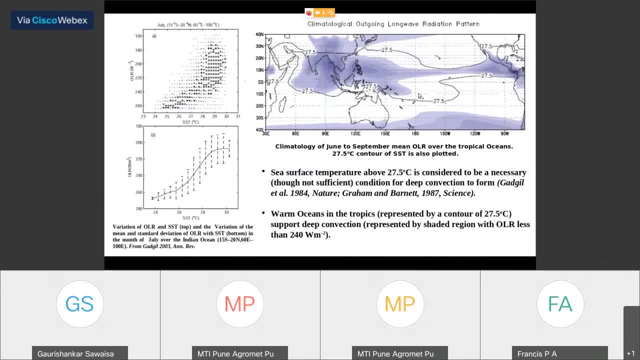 So SST being at 27.5 degree is an essential criteria, but not sufficient. But when you come to the left-hand side, you will see a frequency distribution And what you are going to see is that up to something like 27.5 degree Celsius. 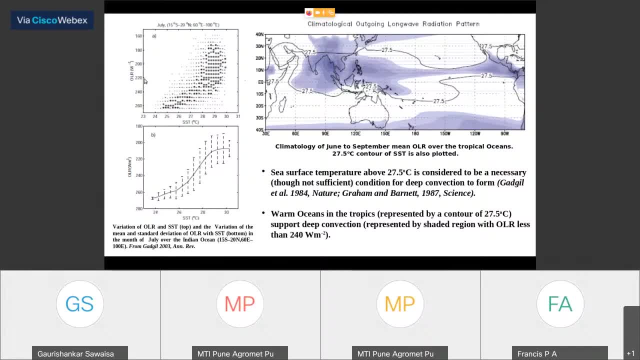 when the SST increases, we can see that there is a gradual decrease in the Euler, which means cloudiness increases. But beyond that you don't have much relationship. Even with higher SST you can have Euler values of the order of 240 or 180, which means that Euler can be anywhere. 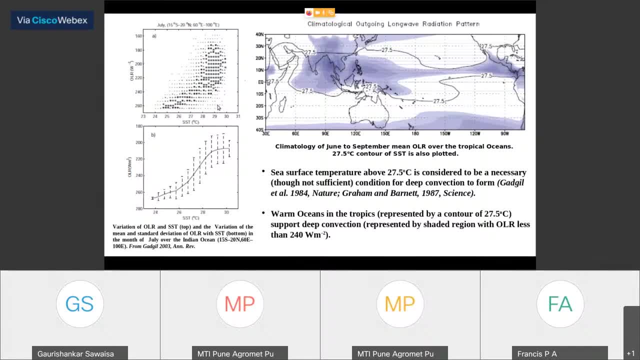 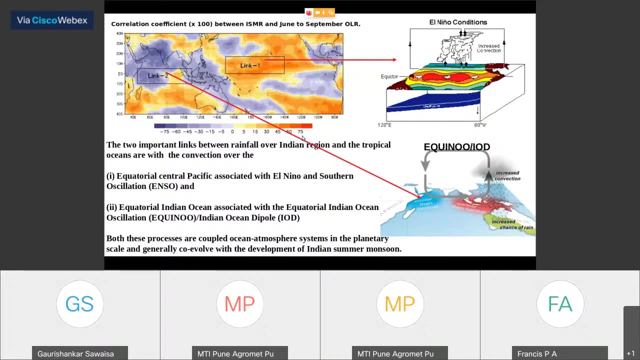 That again says that the warmer oceans are not necessarily the convective regions. but for the convection to happen you need warmer ocean. So this is an important concept when it comes to the ocean. So you can see that the oceans warmer SSTs are going to promote convection. 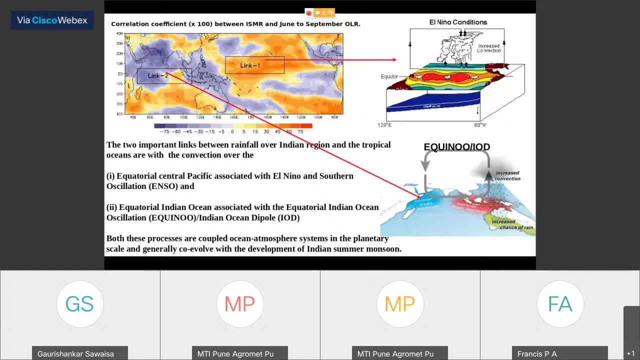 Now, if you want to link the ocean with the monsoon, we need to know how the convective patterns over the warm ocean are related to the monsoon. For this, what I have shown here is a correlation map. What I have taken is that here, June to September mean rainfall as a time. 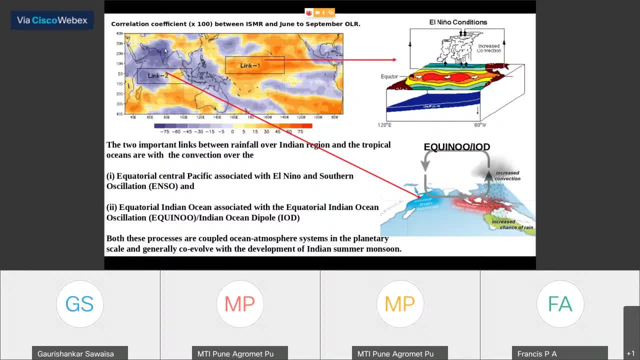 series I have taken over the Indian region and then correlated with Euler everywhere. When you have a positive correlation, that means when rainfall increases over India, Euler also increases. That means when Euler increases means cloudiness decreases. This is a classical example that when the rainfall over India increases, we get less cloudiness over. 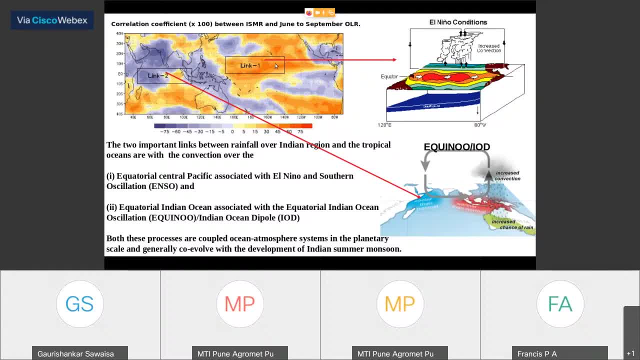 the Central Pacific region And this link is quite known as the El Nino link between El Nino and Indian summer monsoon. You can see that the box which shows the link one is the region where active convection takes place during the El Nino. 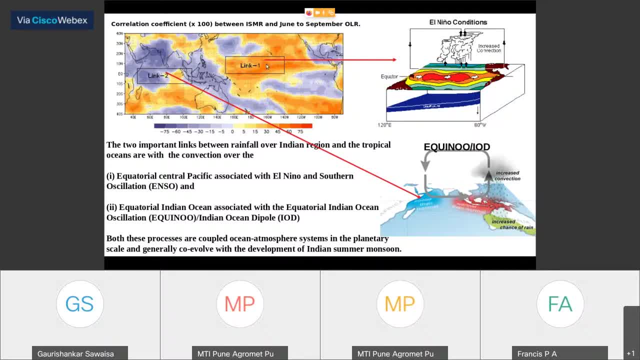 time. So if you have strong convection over this box, it is going to affect the convection over the Indian region. But another link: what you are going to see in this pattern is that, okay, when the rainfall over the Indian region increases, so as it increases over the western. 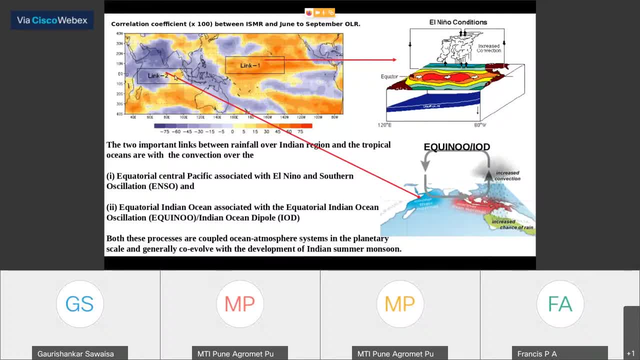 part of the equatorial Indian Ocean, but not same happens over the eastern part. We have a opposite link between rainfall over the Indian region and the convection or rainfall over the eastern region. So we have a situation that okay. rainfall over the western part is good for monsoon. 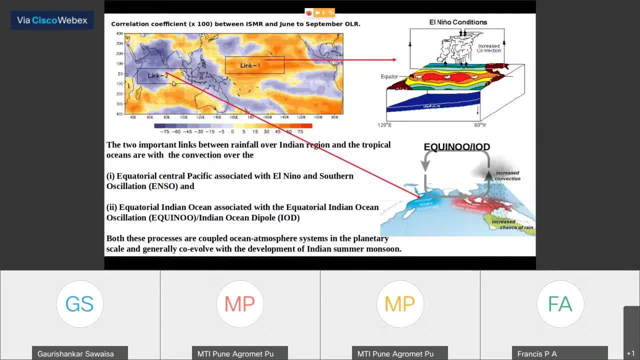 and eastern part is not so good for monsoon. So we have a situation of opposite phases which is going to influence the monsoon, And this link is often called as the equatorial Indian Ocean oscillation link with monsoon, And sometimes these events are co-opted. 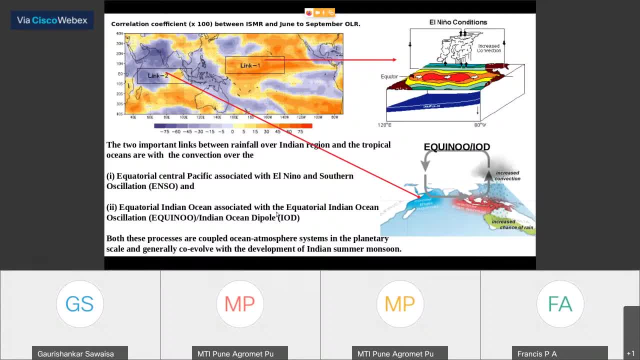 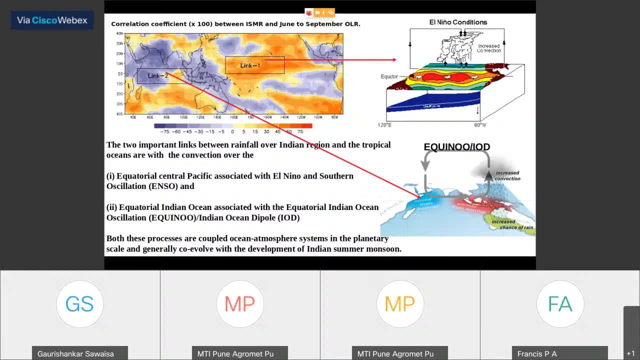 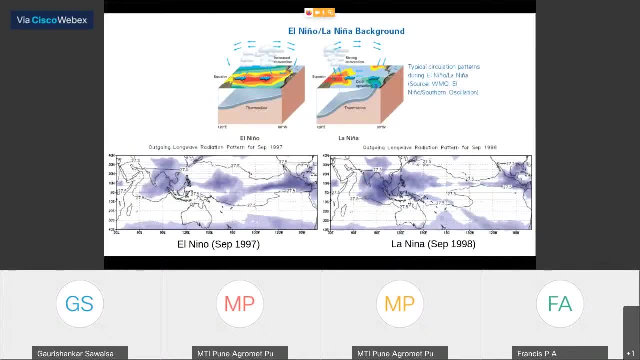 and generally they evolve along with the evolution of the monsoon. That means these systems interact each other. Now to get a little brief on what is El Nino. and we know that El Nino is a situation when the eastern Pacific and the central Pacific is warmer than normal. 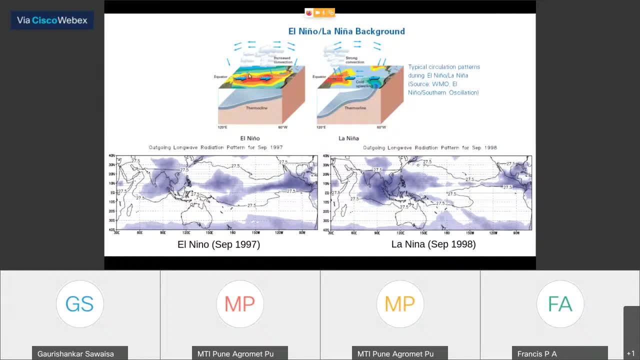 That is what you can see from the more reddish surface over the ocean, And this is associated with slightly deeper thermocline in the eastern part. It is not as deep as the western part, but it is certainly deeper compared to a situation in the La Nina condition. 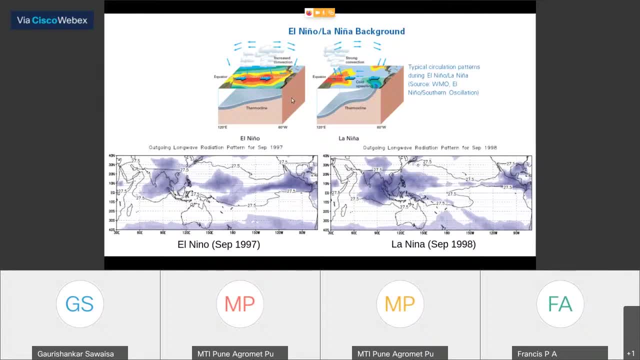 where the thermocline is coming all the way up to the surface, Whereas in the El Nino condition it is slightly in the deeper side And we have good convection happening over the central Pacific during El Nino time and this is how the tropical circulation happens. 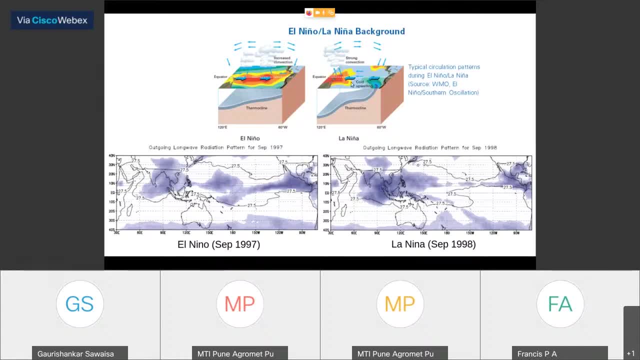 And during the La Nina time we have warmer SST over the western part of the Pacific and cloudiness is intense over the western part. The eastern side is cooler and the thermocline comes almost to the surface, so that cooler water comes to the surface. 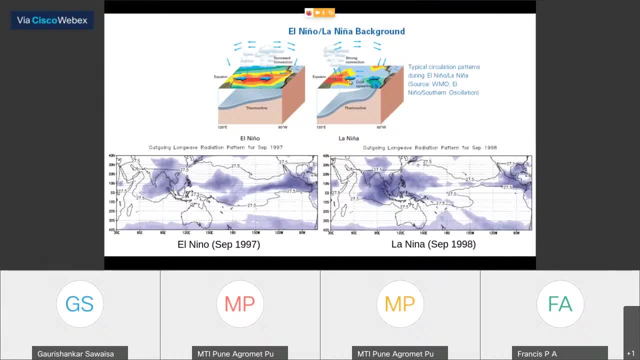 Then we have a easterly wind regime over the tropical portion And we can easily see this from the Euler SST map which is shown in the bottom, And during El Nino time you can see that 27.5 degree isotherm over the tropic is quite fat. There is a considerable amount of area. 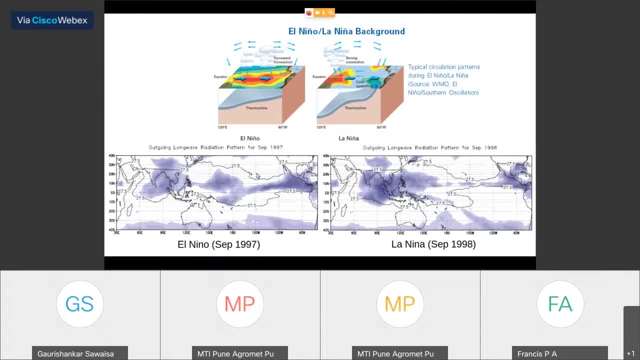 encompassed by this 27.5 degree isotherm in the central Pacific, And this is also associated with increased convection over the central Pacific compared to the western part, Whereas during the La Nina case we can see that the isothermal line, or 27.5 degree isotherm, is quite narrow here and the cloudiness is intermittent. That means not 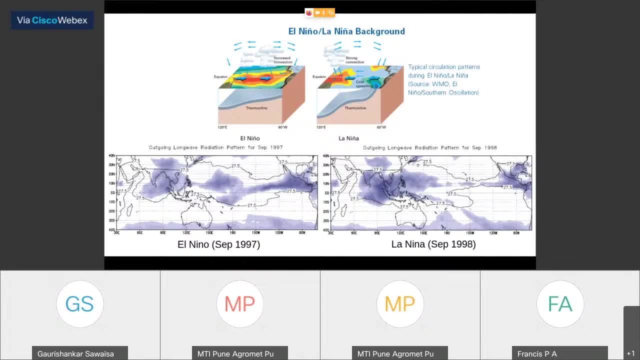 much clouds over the central Pacific, but there is considerable amount of convection over the western part of the Pacific. This is something which we are very familiar in terms of El Nino oscillation, But when it comes to the equatorial Indian Ocean oscillation, 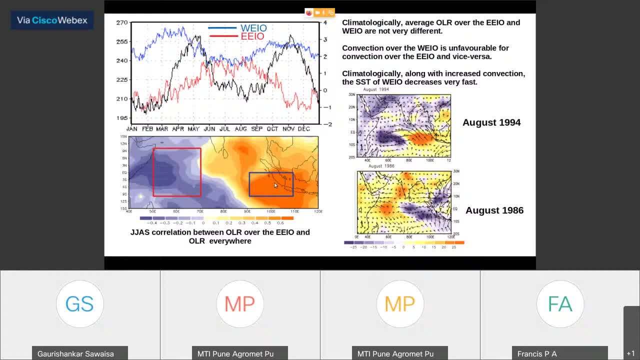 we have a kind of situation where the convection over the western part of the Indian Ocean is unfavorable for the convection over the eastern part And the convection over the eastern part is unfavorable for that over the western part. If you look at the right hand side, 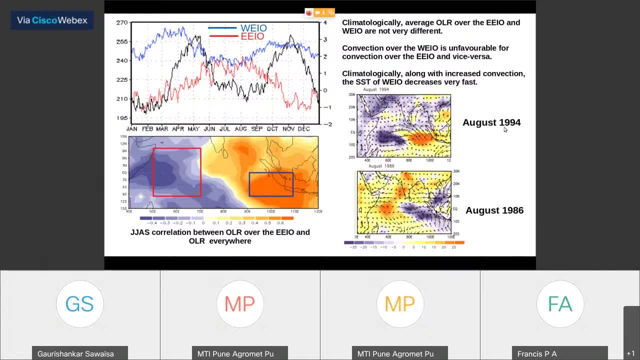 of the slide you will see two cases: 1994 August and 1986 August. These are two opposite phases of equinox. The positive phase is in 1994, where we have excessive convection over the western part. This is Euler anomaly. that means negative. Euler anomaly means more cloudiness. 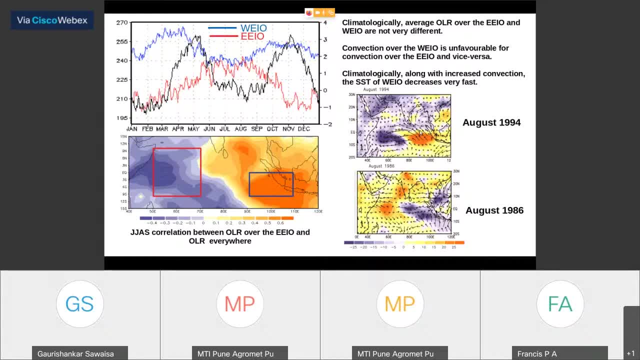 and you can see that the surface winds are blowing from east to west, whereas the eastern part of the equatorial Indian Ocean is less cloudy and this is associated with good convection over the Indian region. The same way, if you go to the 1986 pattern, you have less convection over the 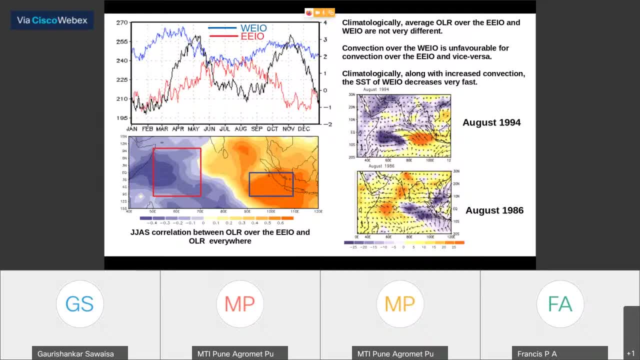 western side good convection over the eastern side, surface winds are very stable and the link between Indian region and the western Indian Ocean are very clean. and this is important because when you have an opposite phase in the convection over the tropical equatorial Indian Ocean, we can. 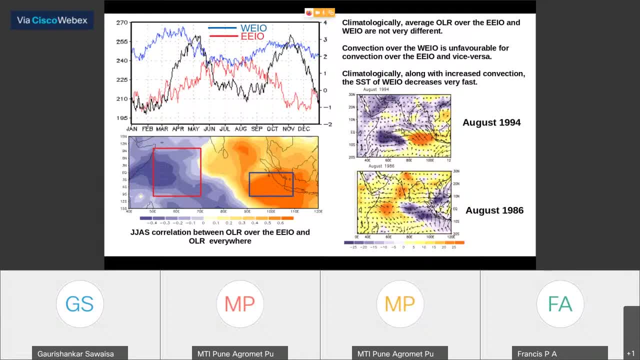 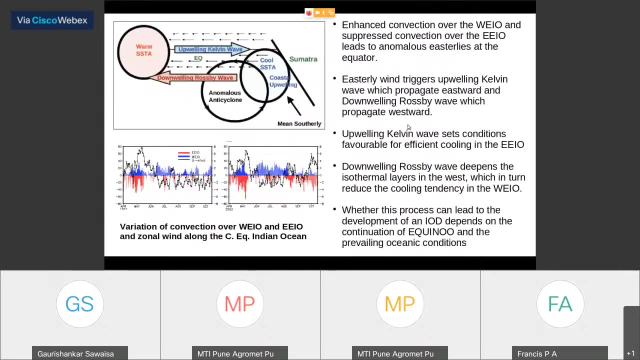 see the reflection of that convection in the equatorial winds also And we generally consider that wind anomaly over the equatorial Indian Ocean, central equatorial Indian Ocean, as a good indicator of equinox. Now there is a lot of ocean dynamics behind the 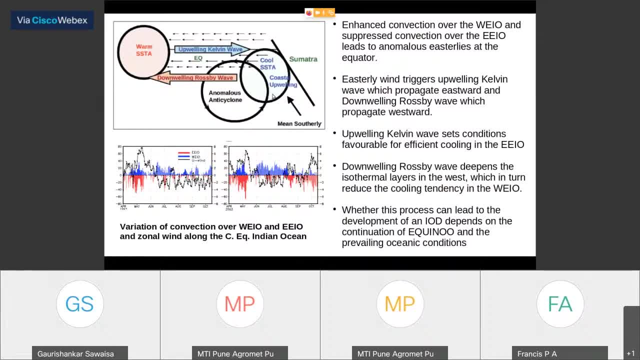 development of equinox and then its subsequent development into Indian Ocean dipole. When we have good convection over the western part, it is going to trigger, it is going to have well, easterlies, as I shown in the picture, And this easterlies can trigger upwelling Kelvin wave which are going to, you know cool, the eastern, 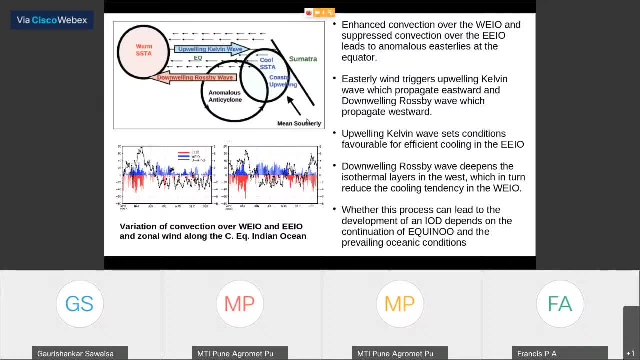 part of the equatorial Indian Ocean, along with the coastal upwelling. So we have a situation: the cooler SSTs over the eastern side. At the same time the easterlies can also trigger downwelling which can go to the west and warm the western equatorial Indian Ocean. So we will eventually get 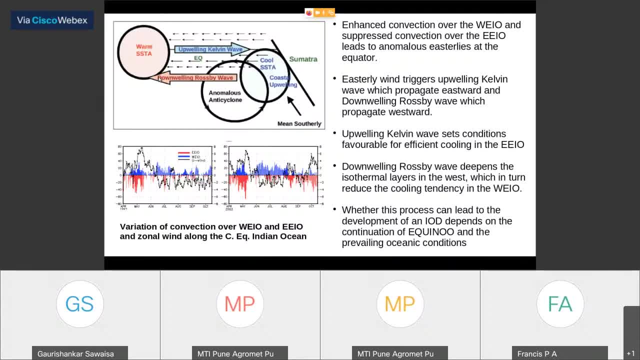 a situation where the western Indian Ocean is warmer than the eastern Indian Ocean, and then we call them as the positive Indian Ocean dipole if it evolves into that level, Otherwise equinox. the convective anomalies can sustain as such without much interaction with or the response from the ocean. It all depends on the preconditioning of ocean, whether ocean is ready to change. That's how the IOD equinox develops further into IOD. 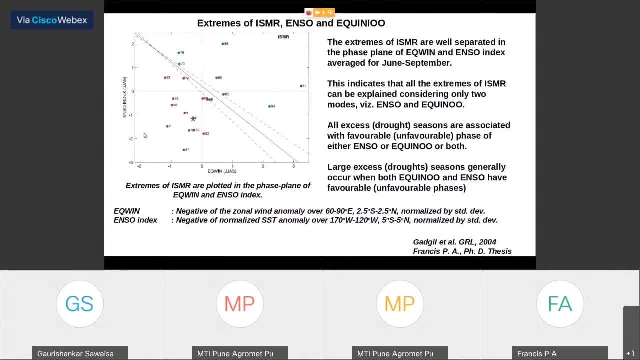 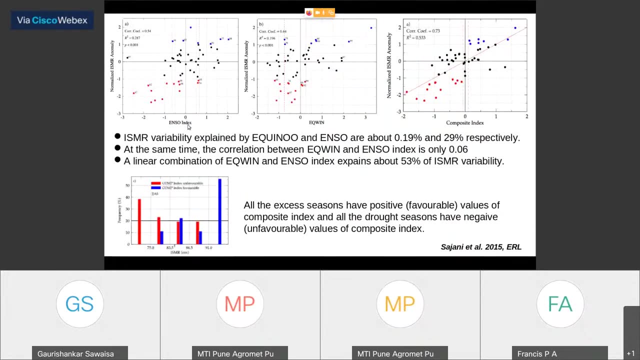 So we have two conditions we have seen. One is the El Nino and the other one is the equinox. We have seen that these two processes or these two phenomenon have links to Indian summer monsoon. And if you look at the individual contribution of these cases, like, okay, if you take an index of ENSO, which is nothing, but I have taken the Nino 3.4 SST anomaly and then multiplied by minus one to make sure that warmer events are bad for monsoon, So negative values are bad for monsoon. So we have two conditions we have seen: One is the El Nino and the other one is the equinox. We have seen that these two processes or these two phenomenon have links to Indian summer monsoon. And if you look at the individual contribution of these cases, like, okay, if you take an index of ENSO, which is nothing, but I have taken the Nino 3.4 SST anomaly and then multiplied by minus one to make sure that warmer events are bad for monsoon, So negative values are bad for monsoon, So negative values are bad. 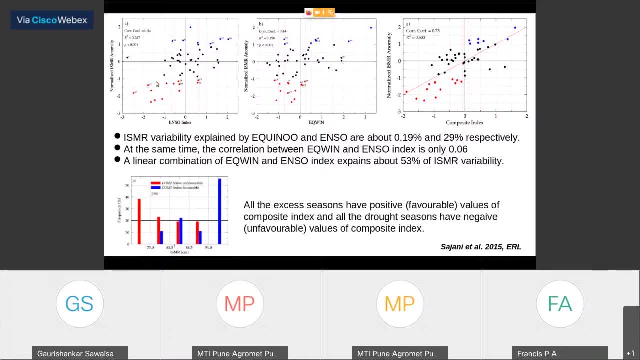 bad. So we can see that when the ENSO index is negative you have large number of droughts, or most of the droughts are happening when the ENSO index is negative, But there are couple of cases when ENSO index is positive also we had droughts. Same way, when the ENSO index is positive, we had mostly excess seasons, but there were couple of excess seasons when the ENSO index was negative. So ENSO is not going to come. 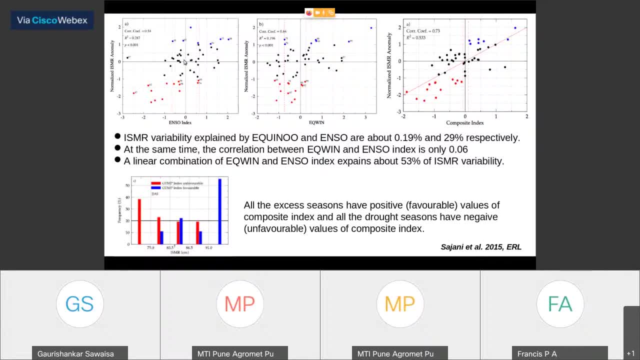 completely explain what happens with the interannual variability of monsoon in terms of their extremes. Same way, if you look at equinox, equinox is also not going to explain everything. We have cases where the positive equinox is associated with droughts and negative equinox associated with excess seasons. So these two are not going to solve individually. but if you put them into a phase plane, the ISMR, into the phase plane of equinox, 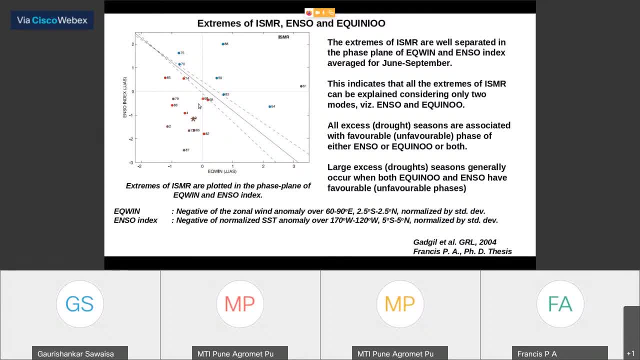 and ENSO. what you are going to see is a clean separation of red dots from the blue dots, and that means when you have both equinox and ENSO index unfavorable or either of them unfavorable, we can get droughts. and when we have both favorable or either of them favorable. 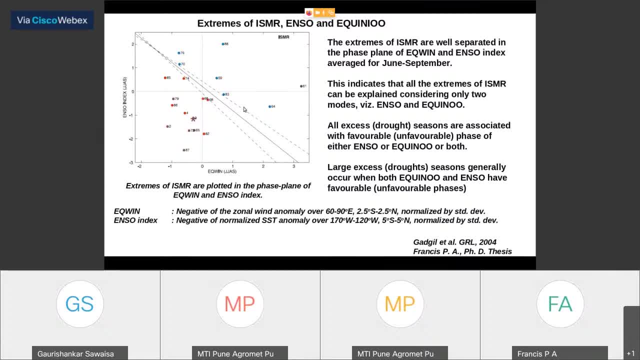 we can get excess seasons. This is very important and we have looked at the statistical significance of this and it's found to be very high. So if you have such two indices and we can see from this slide that both equinox and ENSO are very poorly correlated, You can see that that's very highly. 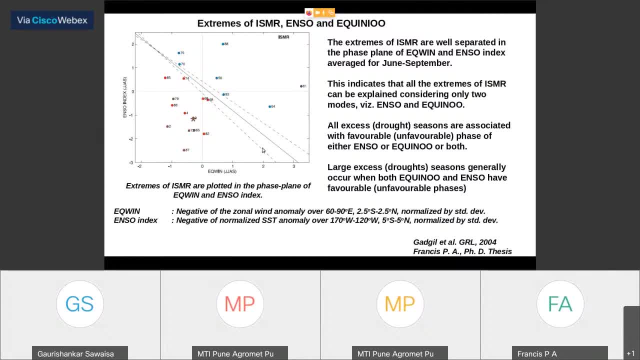 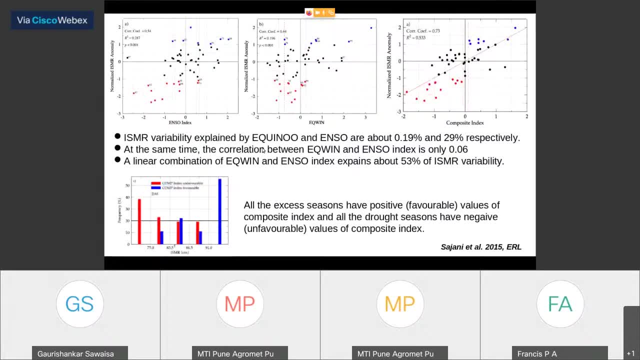 spread. that means correlation values are very low, So this can be considered as two independent modes. as for as equinox and ENSO is concerned, and equinox alone can explain about 19 percent of variability, and INSO can explain about 29 percent of variability of Indian summer monsoon, based on the 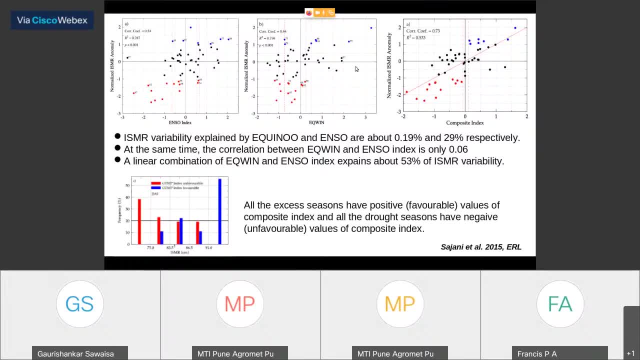 correlation values you see here. but if you put them as a linear combination, then the ENSO index and equinox are put together as a linear combination and construct a composite index. then we can see that all droughts, all red dots you see here are associated with the negative value of composite. 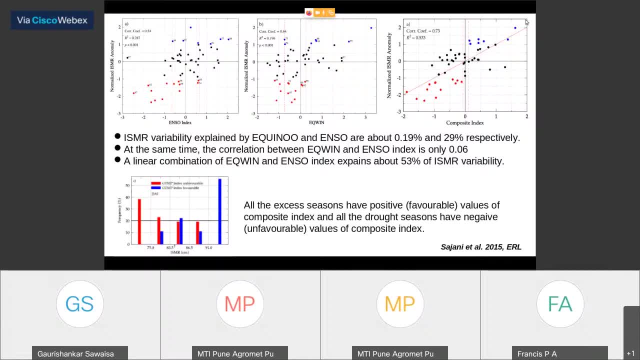 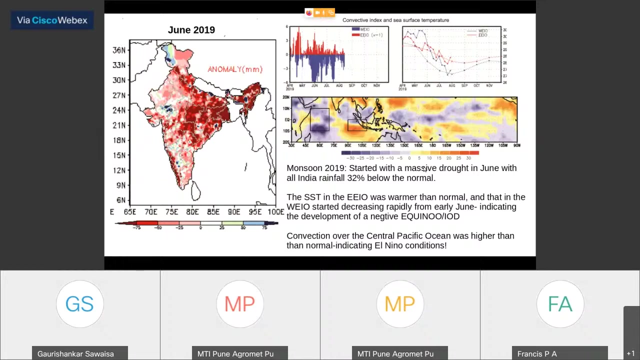 index and all excess seasons are associated with the positive values of composite index, and see that the both these syntaxes put together in a linear combination, it can explain 53 percent of ismr variability, which is very, very substantial. now, with this background knowledge, we were watching the monsoons as they evolve and in a recent case, in june 2019, we have noticed that 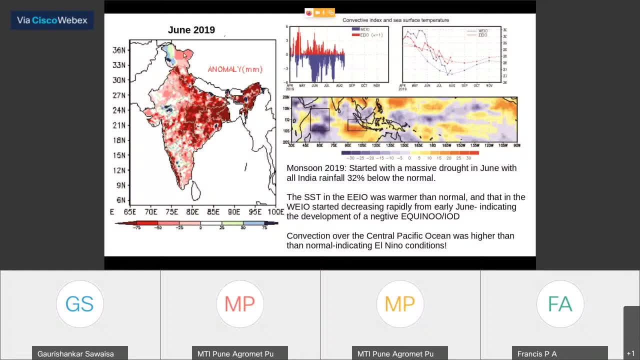 the rainfall anomaly in june over the entire india has was 32 percent below normal in the last few years. when such big anomalies happened in june, they all turned out to be droughts for the season, so these were very important and people started giving more attention to the uh- how the system 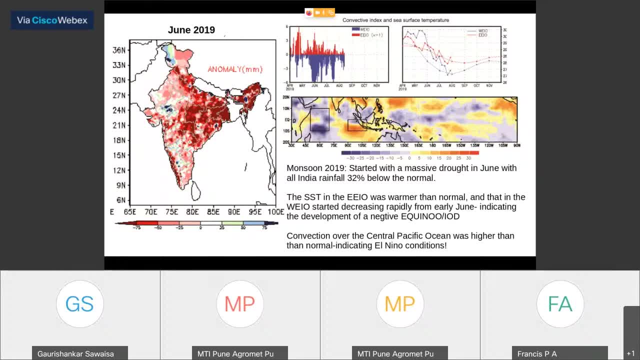 is going to evolve and how the system is going to evolve and how the system is going to evolve in the coming uh months in 2019. another worrying effect was that, when we look at the sea surface temperature evolution- sst evolution- which you will see in the as a time series in the right. 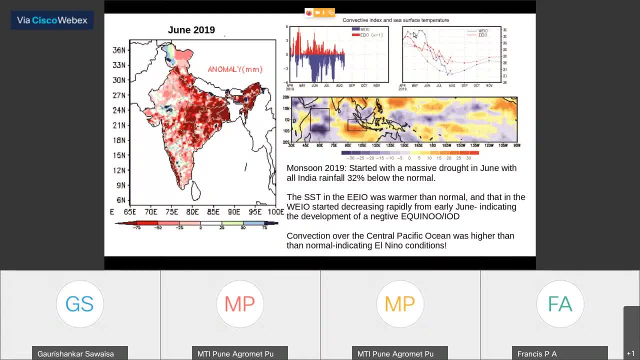 hand side of the slide, you will see a blue curve and a red curve. red curve is for the sst of the eastern generation. blue curve is the sst of the western innovation. you will see that dashed lines on the top of that, which are the long-term means or the climatologies. 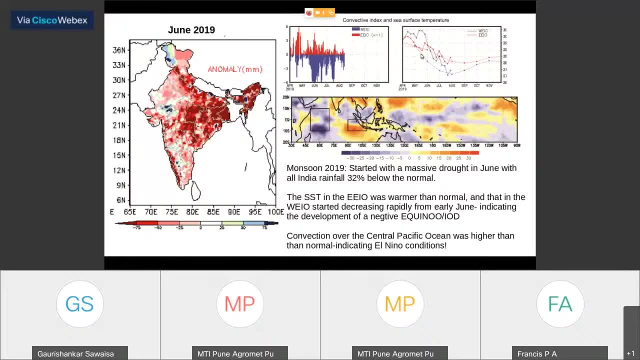 what you can see is that in june 2019, from beginning of june 2018 or late may 2019, the sea surface temperature of the western ocean started decreasing rapidly. it has come to one point of time it has come closer to the climatology or even came below that. at the same time, the ssq of 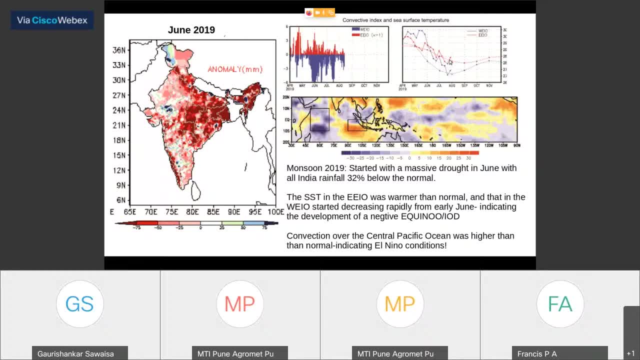 the eastern ocean was remaining warm, more or less close to the climatological values, and this is worrying because this gives an indication of a negative, you know, or a negative iod in the tropical interocean. another worrying effect was that, if you look at the convection over the 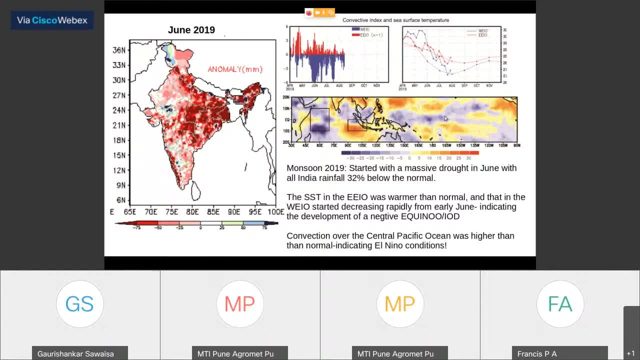 tropical pacific. you can see that the convection over the central pacific was still going on in june and july of 2019, which was giving an indication that lno situation is still continuing. so we have a deadly combination of negative equinox with an lino which can take our monsoon fate very bad. 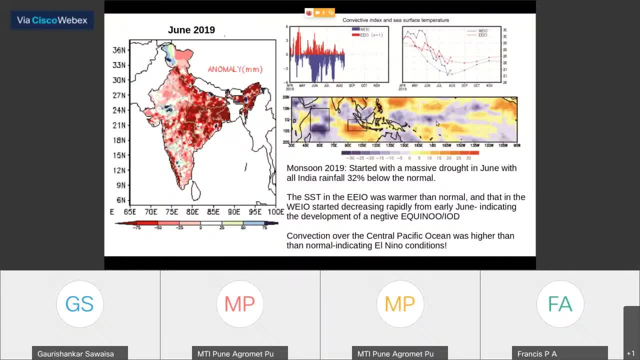 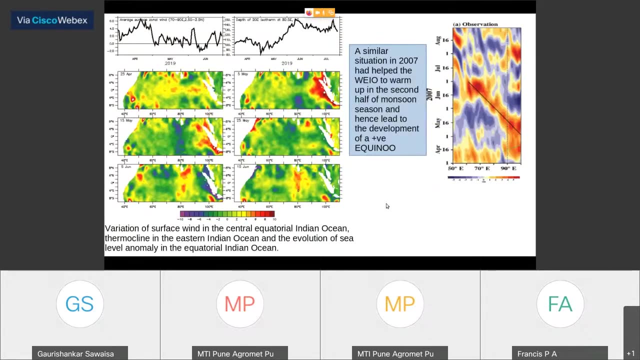 and we can. we have such experience in 2002 and other years. so things were turning out to be very bad in 2019, when we but we kept on watching the events. and what was very interesting in 2019 is that in the left hand side panel you will see. 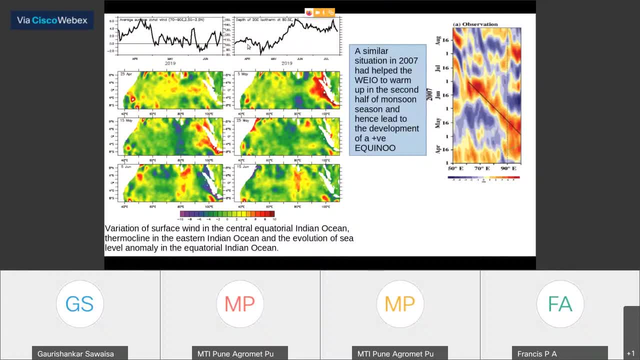 two time series, sort of that. the right hand side time series is the depth of 20 degree isotherm at 80.5 degrees just south of sri lanka, and this was observed by a moored buida and you can see that the depth of 20 degree isotherm is more like the depth of thermocline in the ocean, where up to which 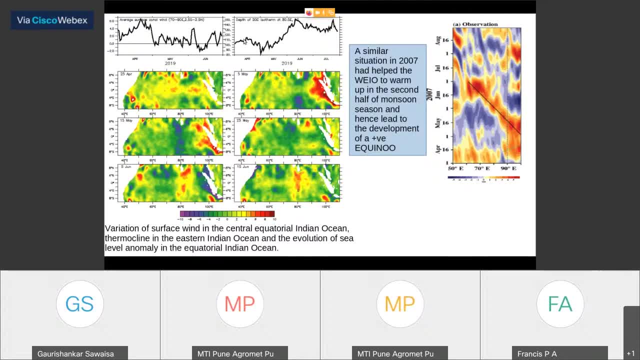 we have the warmer waters and the thermocline was quite shallow uh in the beginning of may, but as the season progressed we can see that the thermocline started increasing uh deeply and we can see that it has gone up to something like 140- 150 meters by early june. this was associated with a kind of 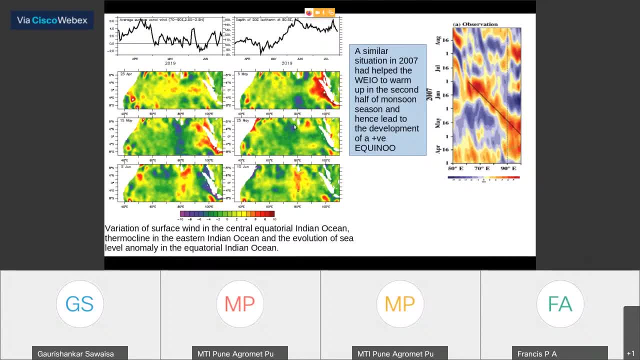 sea level anomalies which you see in the sequence panel, uh sequence figure. in the below panels you will see the sea level anomaly on 25th april, then 5th may, 15th may, 25th may, 5th june and 15th june. what you see is that on 25th april you can see that there is a positive 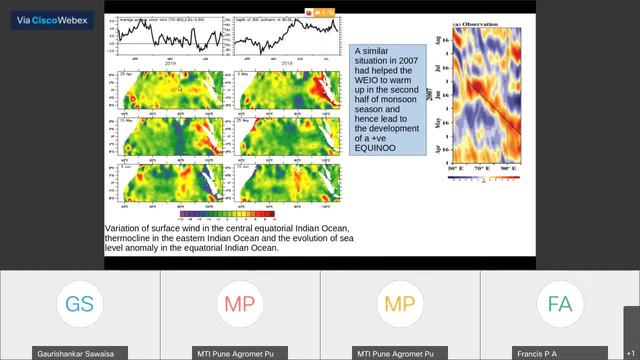 anomaly of sea level, anomaly in the central and eastern indian ocean, tropical indian ocean, which has further gone to the east, hugging to the cost of sumatra, and then started moving out both in the southern and northern hemisphere, and then it started further moving away from the coast as 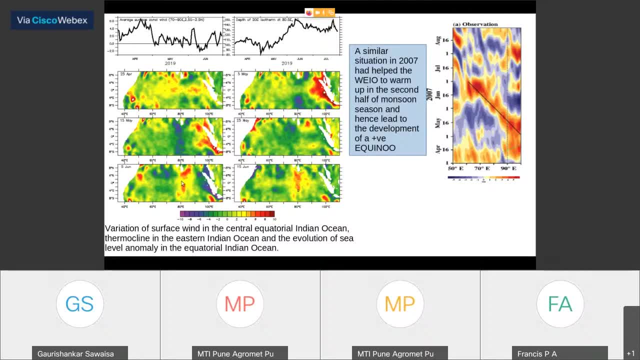 and by 5th june you can see that they have come all the way to down, uh deep, of sri lanka and then south of it. this is where you saw that deeper thermocline in the buoy observation and from our experience we know that the situation is something like a westward propagating. 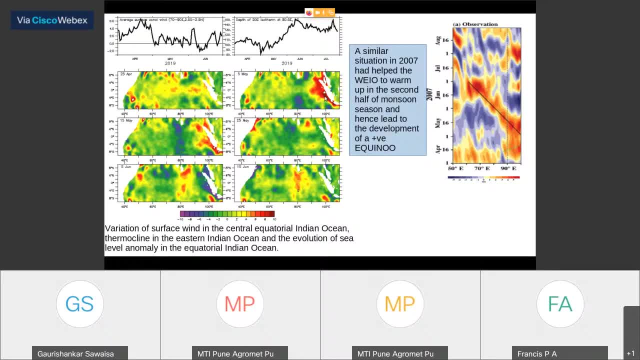 downwelling raspy wave which has in fact come from the eastern boundary of the equatorial indian ocean, and we know that once this uh raspy wave is formed, it is going to move further westward, deepen the thermocline in the western side further. 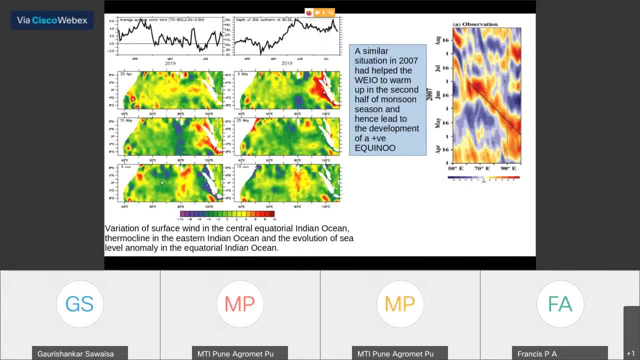 and this can arrest the cooling in the western ocean. so this was a speculation, but there was a reason behind that, because in 2007 a similar case happened and you can see the how the sea level anomaly propagated to the west. this is the observed sea level anomaly and the red patch with 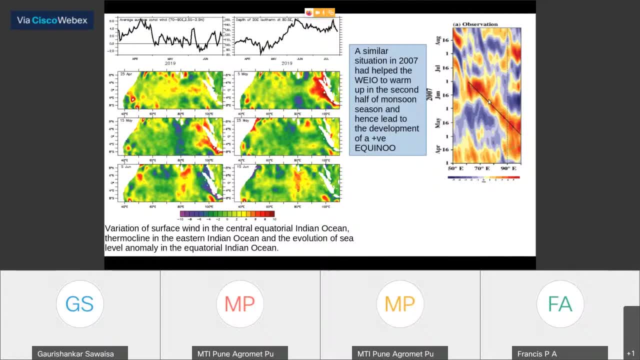 a black line over the top of that is actually is a black line over the top of that is actually is a a westward propagating raspy wave and we could see that in 2007 when this raspy wave reached the western denotian. it has actually arrested the cooling of western denotian and that gave a clear 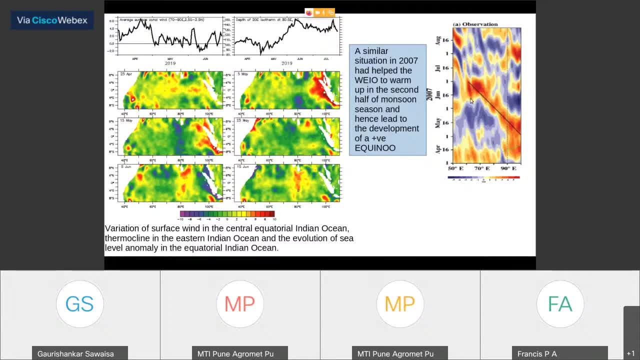 background for the positive equinox to form further, and that became a full-fledged positive equinox in 2007, and then the monsoon became very, very good in 2007.. so we were anticipating a similar situation in 2019, even though situation in uh by end of july was not very good looking. but 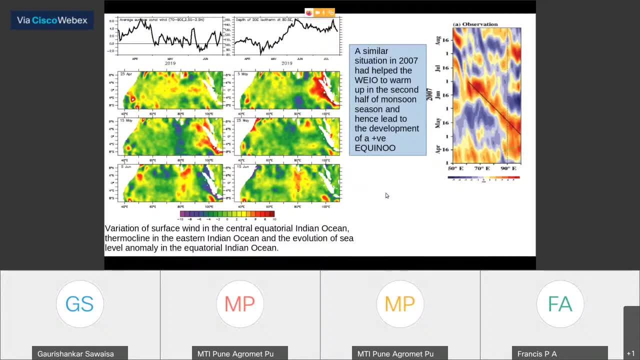 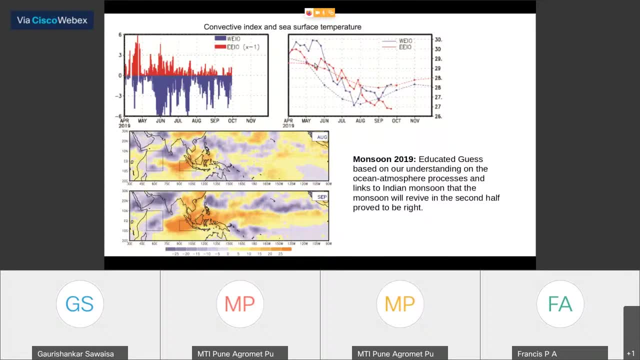 only hope we had was that this raspy wave is going to do the same thing, what we had seen in 2007.. and when we, when we put our educated guess and then later came back and validated that we were- um, you know- proved to be right, you can see that this is where we stopped our observations when we came and said that look. 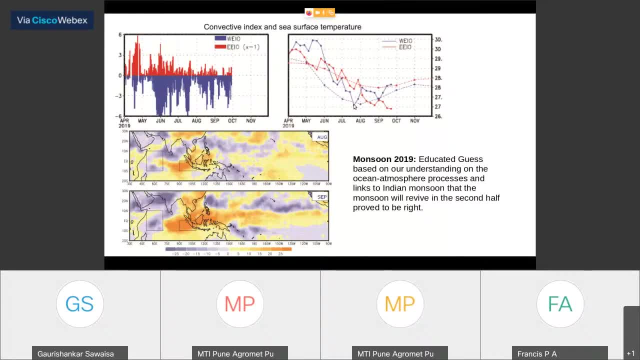 there is a raspy wave coming and it is likely to deepen the thermocline in the western denotian and arrest the cooling there, so it can trigger a positive equinox. and when we came back later and looked at the sst in the west indian ocean you can see. 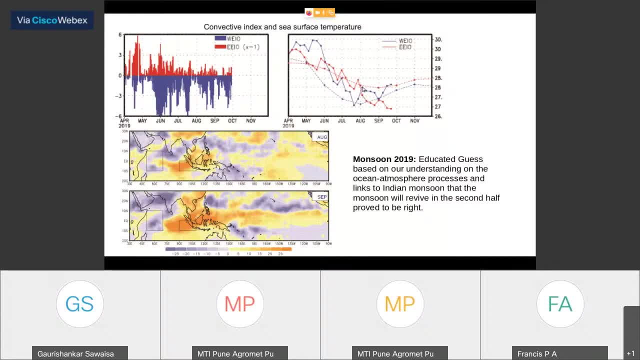 the sst started increasing substantially. it has gone all the way up to 28 degrees celsius by early august and with that the eastern denotian started cooling. a perfect combination for a positive- you know, positive- iod to develop and a good rainfall to follow. and this is what happened. 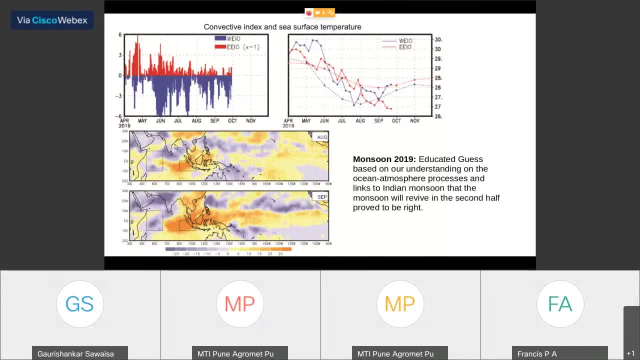 in the bottom panels you will see the oiler anomaly patterns of august and september. you will see a positive, you know, with enhanced convection over the western, denotian less convection over the eastern, denotian good rain over the indian region, and same thing continued. 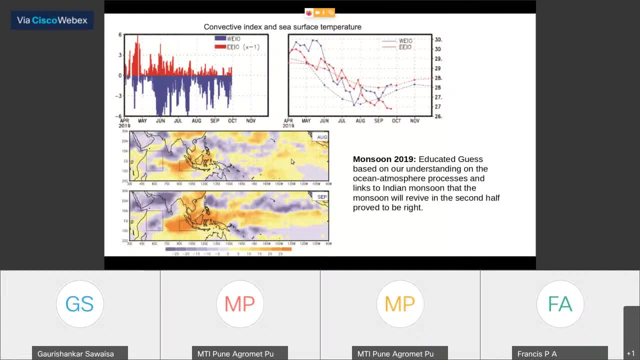 with much more intensity in september. added to that, the signal of el nino in the central pacific vanished by the time. so, ultimately, 2019 turned out to be a good monsoon, despite having a below normal rainfall of massive below normal rainfall in june. this observation 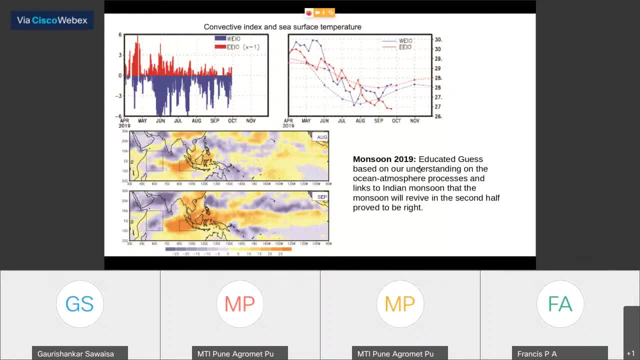 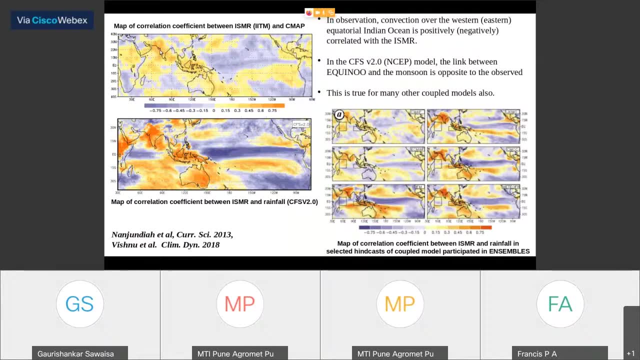 we have and the understanding we have should be translated into the models for a forecast and how much we have succeeded in that. so what i have again shown here: a correlation map of rainfall over the indian region, or ismr. we can say to a rainfall everywhere this time i have 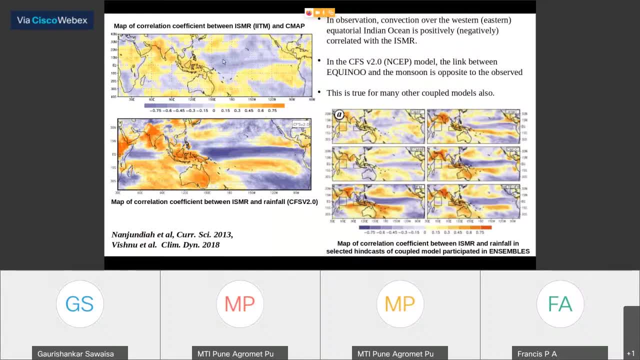 taken rainfall instead of oiler. so opposite correlation is really opposite. that means when the rainfall over indian region increases, rainfall over the central pacific decreases. this is very clean from the observation and also we can see an opposite phase in the equatorial indian ocean. rainfall over the indian region is oppositely correlated to that in the eastern. 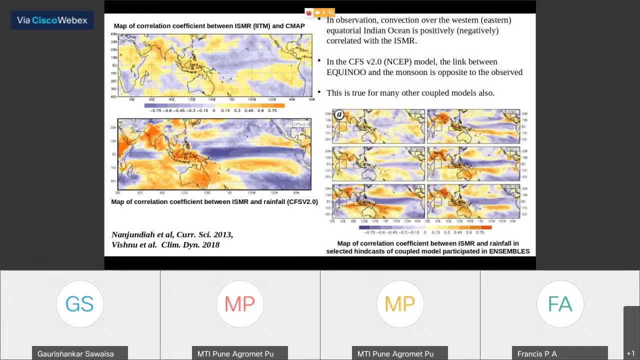 region of the tropical denotian and to the positively correlated to the western indian indian ocean, with convection over the or rainfall over the western denotian. now this combination, are we getting in the models? what i have shown in the bottom panel is the same thing i reproduce from cfs. 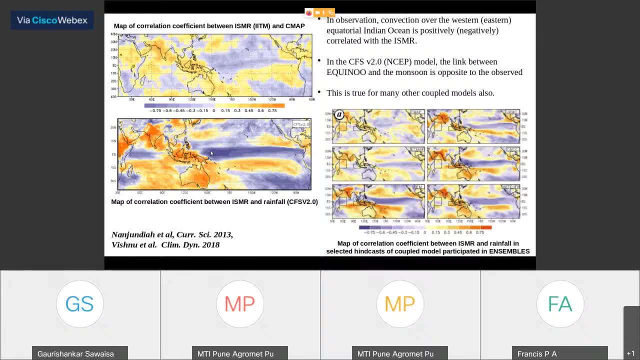 two models and you can see that of course, the pacific system has been captured. you have opposite relationship between rainfall over india and the central pacific and this was very well captured and we can see that it's a bit more intense than what we expected. but if you look at the, the map over the 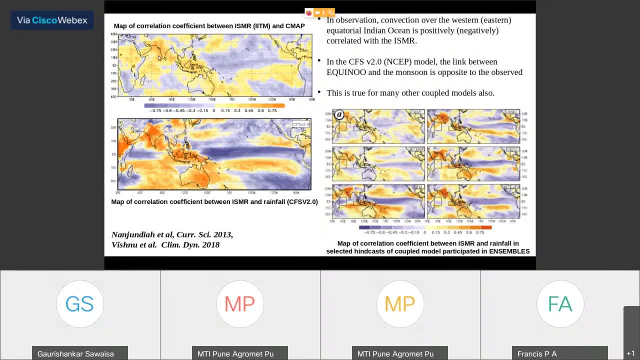 indian region. this is exactly opposite what we saw in the observation. we don't get the same correlation between the western denotian or opposite correlation to the eastern denotian. this is a problem. and this is not a problem only for the um, only for the cfs2, it's a problem for many of the ocean. 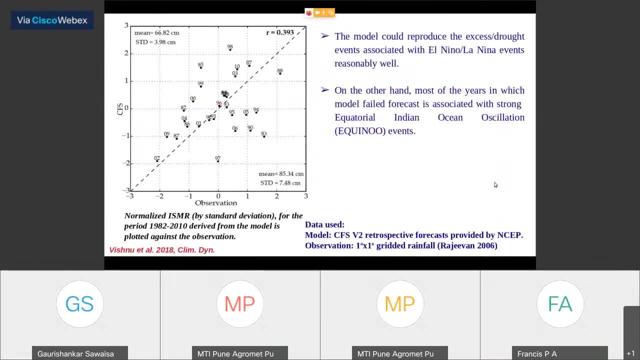 atmosphere coupled models. now, when we look at more carefully with the model, you will see that certain years, like 1983, 1997 years, the rainfall captured or the reproduced by the model are not as good as we should have or what we found in observation, for example. 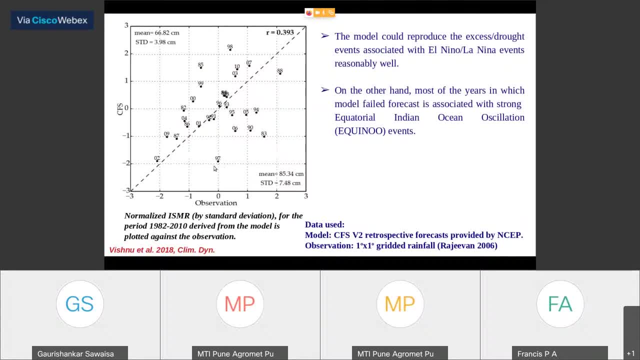 1997. the observation shows no post anomaly in uh all india rainfall. that means the ismr anomaly was close to zero. but cfs model predicted something like minus two standard deviation rainfall, same as in 1983. whereas we expected, or we were, we experienced an above normal excess season in 83. 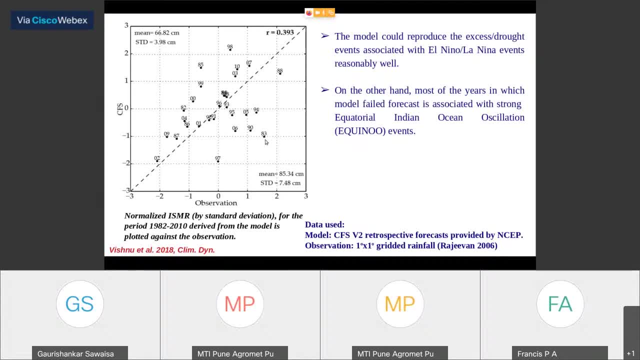 but what we predicted by cfs was negative anomaly. so these are concerns and these are. we know that 83 and 97 are associated with equinox, so the models have difficulty in getting the link between equinox and monsoon right, and this continues now also. 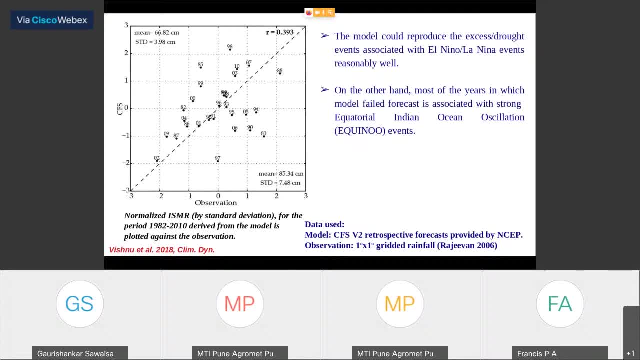 and that's why we are not able to get the equinox based monsoon extremes right in the models. at the same time, when we have strong leno, we get its influence on the model and we get things right. so, um, i will just quickly go over this slide, because this is something which is 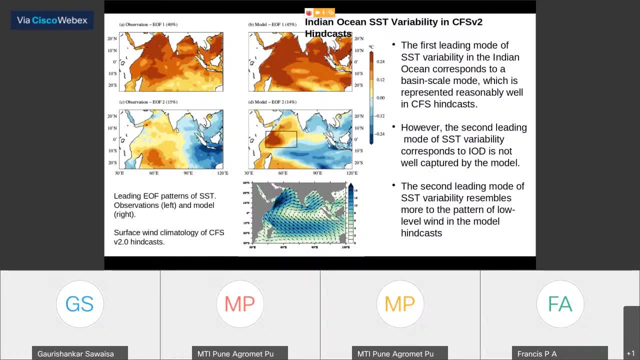 showing the how good the model is reproducing the indian ocean variability in terms of, you know, empirical orthogonal function patterns. and we can see that the first pattern is captured very well by the model observation in the left side and the model in the right hand side. the basin scale- warming or cooling- has been captured very. 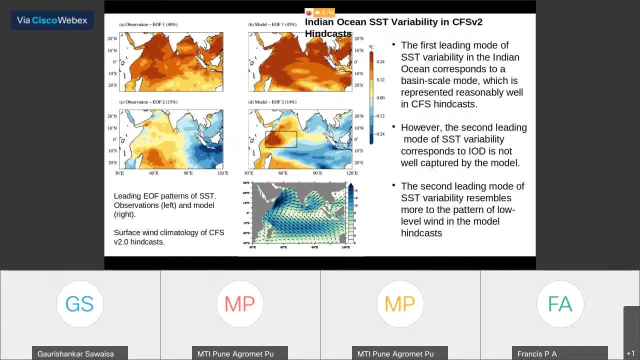 well by the model, but the second mode, which is considered to be the indian ocean dipole, is not well captured. what we find for the model is a region where, in the east western indian ocean, having a very high variability, and this is extending to the eastern side, along with the flow of monsoon, which i have shown in the bottom. 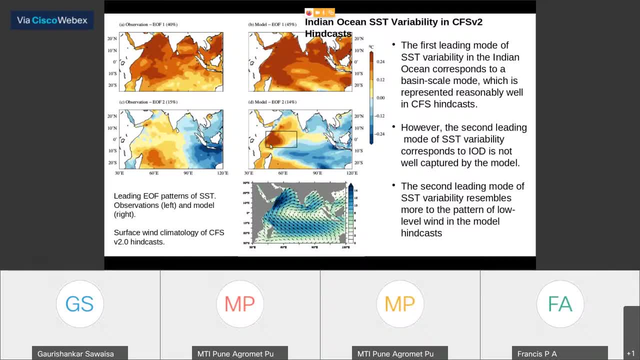 so monsoon winds are carrying these anomalies, so this is not surprising that when in a normal condition, when we have strong winds along the somali coast, it's going to create a building situation and this upheld cold water are going to be transported to the eastern side through the monsoon currents, and that's what we see in this one. 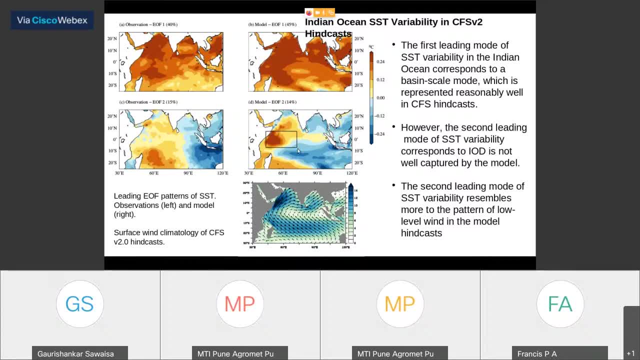 so the ocean dynamics does not seems to have played a role in getting this anomaly in the indian ocean, at least for the second mode of the variability. but first mode comes right. so iod is not well simulated by the model and further we have shown that this is just because the 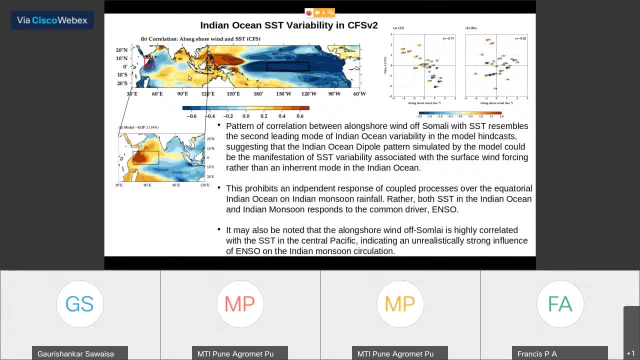 indian ocean circulation in the model is completely driven by the pacific circulation. so if you have an el nino, it's going to dictate the monsoon flow and irrespective of whether you have an internal um mechanism or the indian ocean dynamics in the observation for the actual situation, 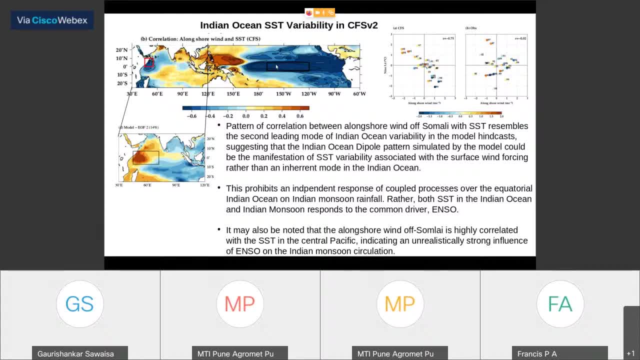 the model is not going to reproduce any of those things. model will just behave to what happens over the pacific. and we also know that that link between the indian monsoon and the pacific uh system, that el nino, is very strong. so we will have a situation that el nino dictating the indian. 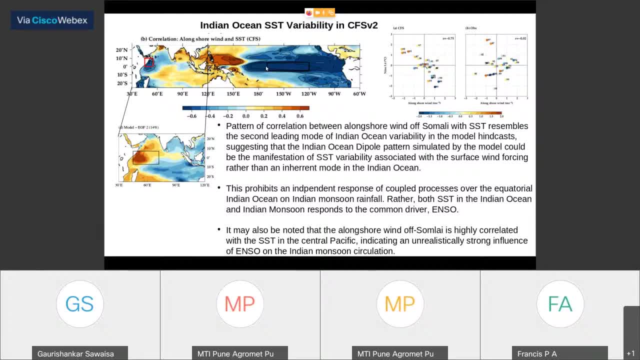 ocean circulation, indian ocean ssd pattern, as well as the indian monsoon rainfall, and which are going to be completely opposite in phase, and hence we will not get the link between and so and el a, so you know, or equine so derived in the model. but there are two curves. one one is the full correlation and another one is a partial. 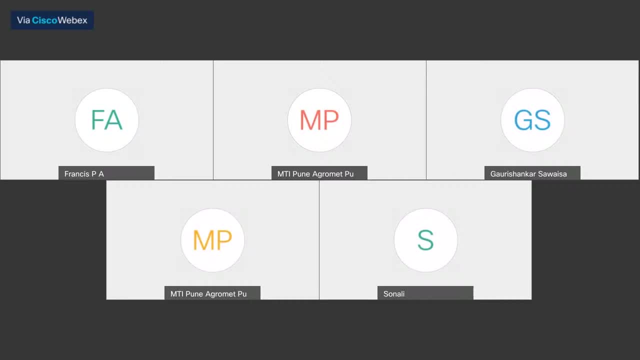 correlation by removing the effect of el nino, because we know that elena is influencing the indian ocean circulation quite a bit. suppose we remove it. statistically, what will happen so if we are not removing it? what we see in the extreme right is the observation. it should be a. 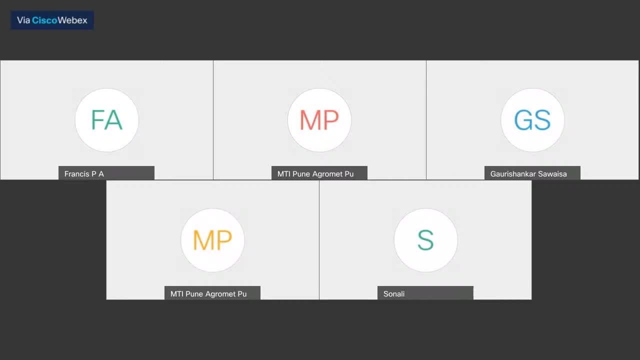 positive correlation of about 0.4. but what we are going to get in the most of these cases is negative correlation, and that we expected from the previous slides. but once we reduce the effect of impact of leno, we started getting positive correlation. that's the red sticks, which is 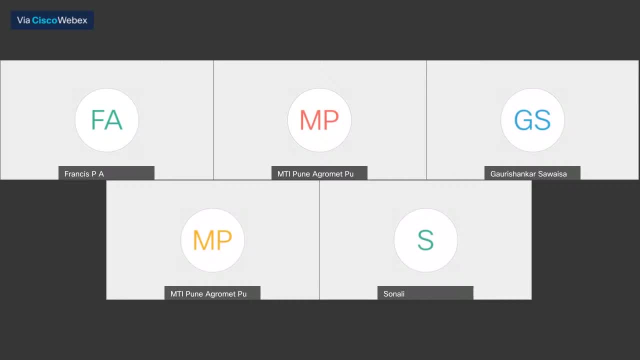 sticking upward. so we are, uh, having a situation. we have having models which can do well, provided the, in fact, impact of, and so are somehow brought down, or we have to scale down the impact of, and so in these couple models, to get the indian ocean variable to take a role and dictate the indian monsoon in the coupled models. so to summarize, uh, i will. i. 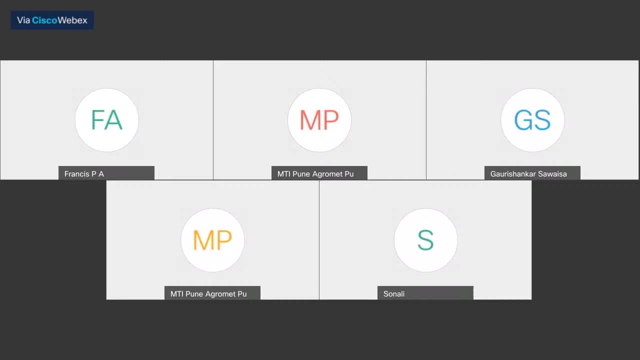 have put a few blood points. uh, we know that the internal variation of indian summer monsoon has close links to the ocean atmosphere processing the indian ocean and the pacific ocean, and it's important that we observe these features so that we can get a good clue. 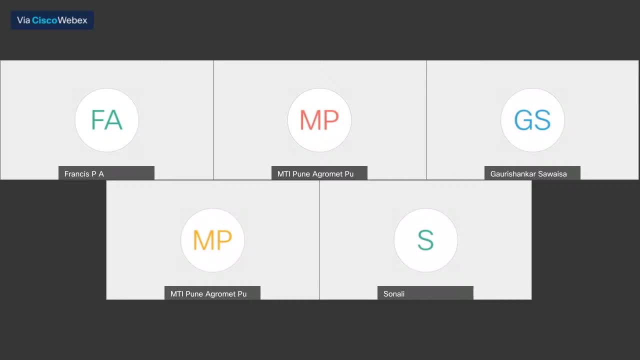 on how it's going to evolve, like what we happened to have in 2019. at the same time, couple models have to be improved. they are good in simulating the ensuing fitment soon, but they have to be proved or tuned better to get the equinox link also right. probably this can be. 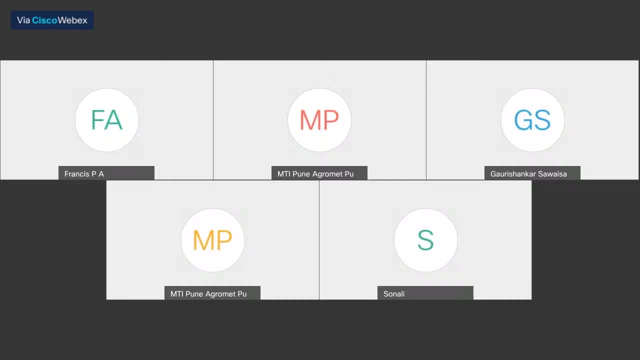 done by focused effort in to look, by looking at the physical relationship between these and the couple models. what we found so far is that, if you know, or iod comes as a response of nso, then it can be used for calculation over the equatorial indian ocean. okay, thank you. 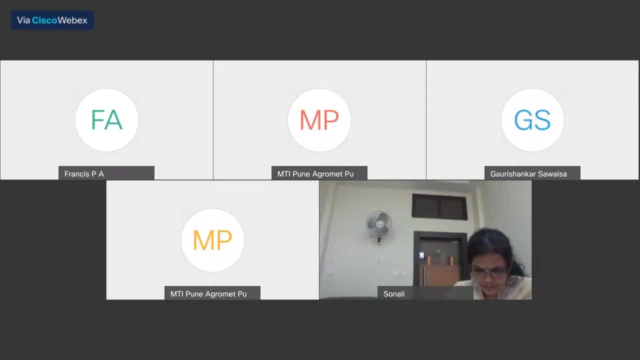 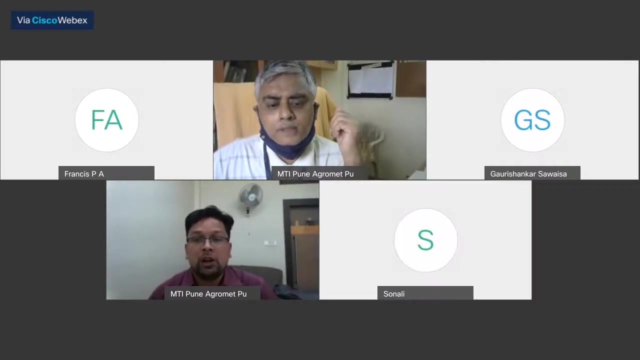 thank you, dr francis sir, for your interesting and informative lecture. now i would like to request dr critical sir, scientist c, to give vote of thanks. at the outset i wish to express my sincere thanks to honorable dgm imd for kindly interested upon this assignment to mti for building community capacity in the field of weather and allied. 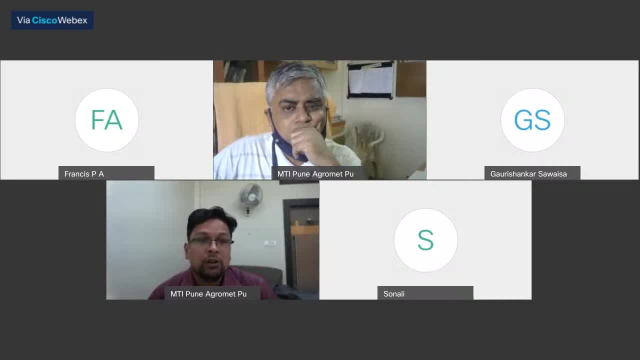 services. it is my privilege to propose a vote of thanks on behalf of metrological training institute. i would like to express our sincere thanks to the mti for providing us with the opportunity to present our work to the public and to the public, and to the public and to the public.